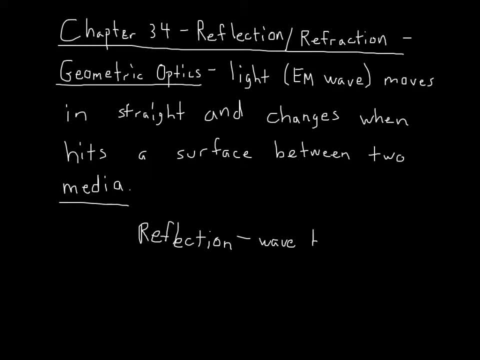 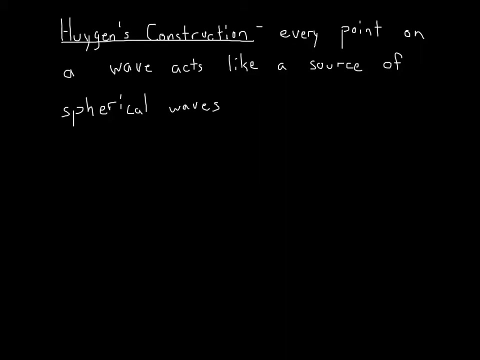 bounces back Or with refraction, So I can have reflection or refraction, And refraction is when a wave bends, And we're going to talk about each of these in a little bit more detail, And something that might come in useful as we're discussing reflection and refraction is this concept. 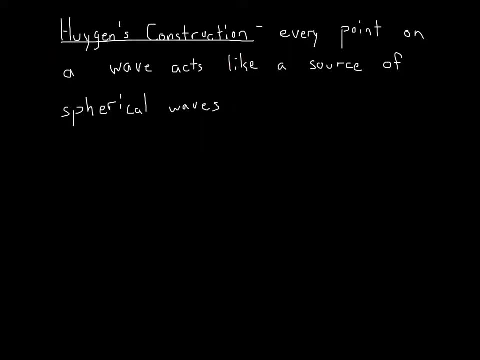 of Huygens' construction. Huygens' construction of how light actually works, how a wave works, And what Huygens said was that every point on a wave acts like a source of spherical waves. So this sounds very strange, sounds a little bit abstract, but the way I think. 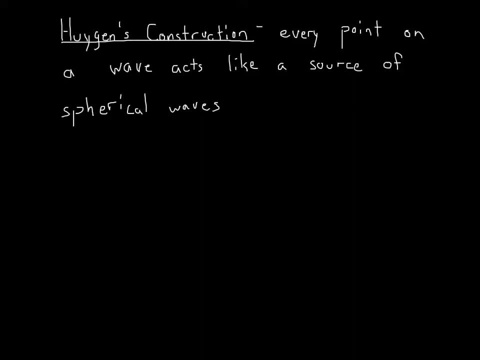 of it is, every point on a wave is like a pebble. So I take a pebble and I drop it into the water. When you do that, you see ripples that come out. These ripples come out in big circles. These circles are the spherical waves that are emanating from this central point. So 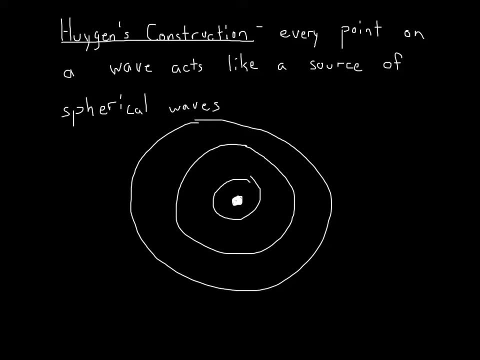 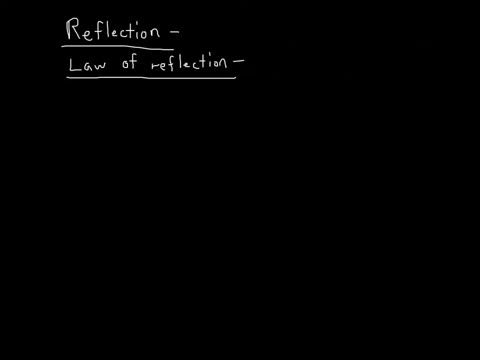 what we do is we imagine that every point on a wave is like this little pebble and it creates a spherical wave that moves outwards, away from it, Like dropping a pebble into a pond. So in discussing how light moves in geometric optics, the places that we usually start is 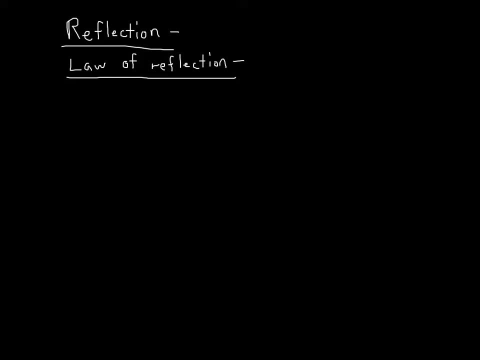 discussing with reflection And, in particular, we talk about the law of reflection. So let's say I have a medium that separates two surfaces. Maybe I have air up here and I'm bouncing some light off the ground and the ground is maybe covered with snow. Okay, so I have two. 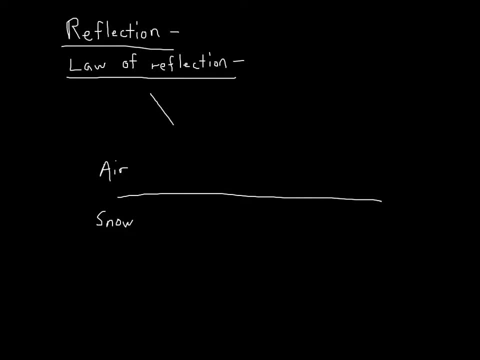 different surfaces And when a light wave comes in. Okay, so I have two different surfaces And when a light wave comes in, I'm going to draw that like a little arrow And I'm going to call this a specific name. I'm going to call this an incident wave. So that's the source of my light ray And what? 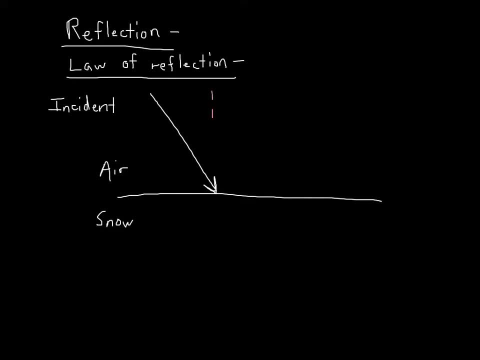 I can do is I can draw a nice perpendicular line separating my surfaces, Drawing a line perpendicular to the two surfaces, And this light is going to be absorbed by the ground but some of it is going to bounce off. And I'm going to draw that bouncing light Bouncing off of whatever surface it hits. 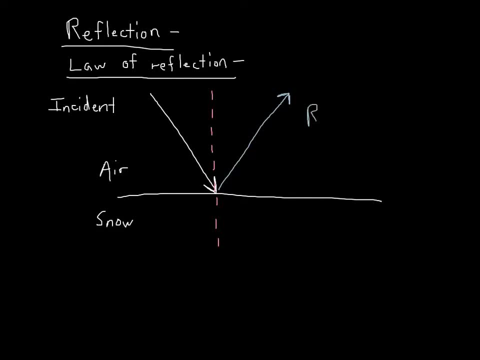 And we're going to call this the reflection wave. Something we should notice is that when I'm drawing the waves in geometric optics, I'm drawing them as arrows. I don't try to put in the wave-like shape. That just confuses things. But we need to understand that these 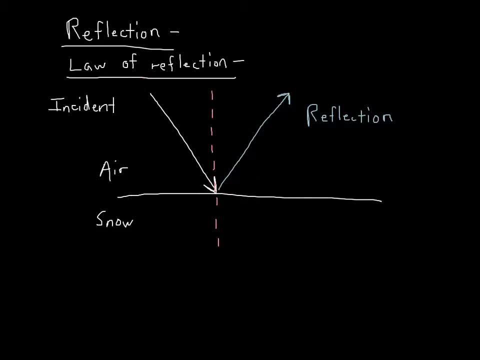 arrows represent actual light waves, And something I can do here is I can draw the angle between the vertical perpendicular, that red line, and the incident ray- I'm going to call that theta. And then I can draw the angle between the reflected ray and that vertical perpendicular, that red line, And I can call 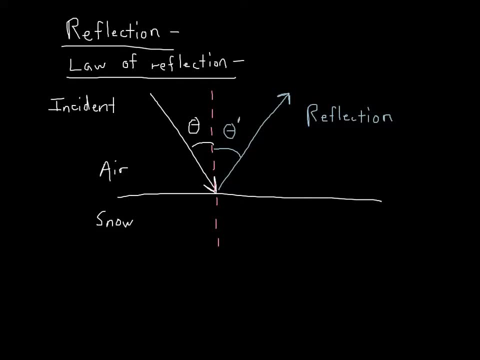 it, theta prime. And what the law of reflection does is it takes the angle between the vertical perpendicular, that red line and the incident ray. And what the law of reflection tells us is that the angle of incidence theta is equal to the angle of reflection, theta prime. 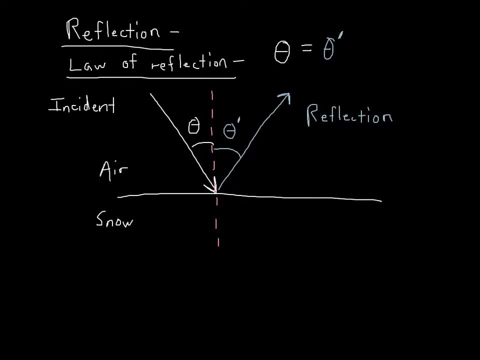 So that is the law of reflection: The angle of incidence is equal to the angle of reflection, Incident angle is equal to reflected angle And it's all relative to the vertical perpendicular reflection To your two surfaces. So we'll return to discussing reflection a little bit later, But for now let's move. 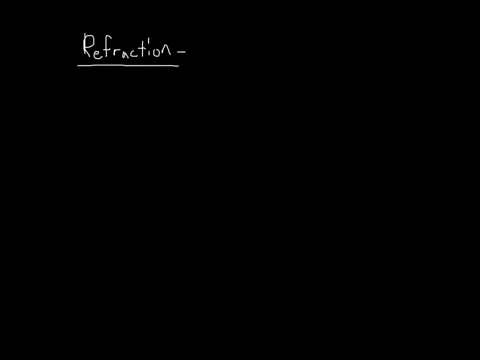 on and talk about what refraction is. And refraction is when light bends and, in essence, this bending is actually the light changing speed. So refraction is when light bends, when light hits surface, And we know that refraction is light bends when it hits a surface. 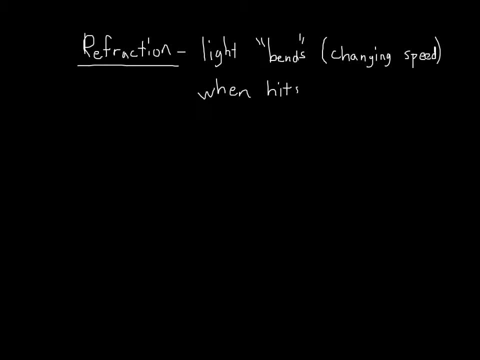 So refraction is when light hits surface and in essence, the light bending speed is exactly like the result. So let's look at reflection and refraction. Refraction is refraction's bending speed. If reflection were bending, then the angle would be equal to Democrat score. 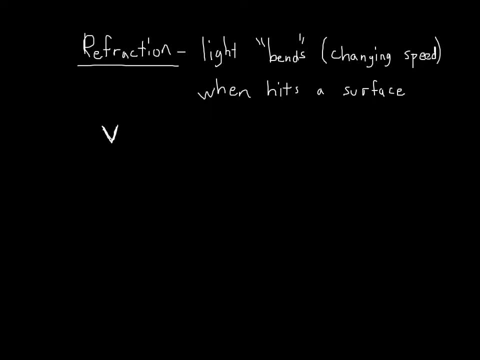 Refraction is when electricity is moving around. Refraction is: refraction is when electricity is moving around. Euclidean reflection: Correct, Ok, Refraction isonst �m awaits Nit mystery, the well-known speed of light c. this is the speed of light in a vacuum. so how? 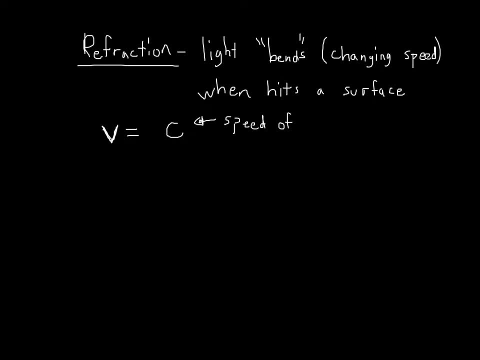 fast light is going in a vacuum divided by this letter n, where here our n is something called the index of refraction. And here we see that refraction word coming up again. Our n varies. For a vacuum it's equal to 1, and otherwise the n is always going to be greater than 1.. 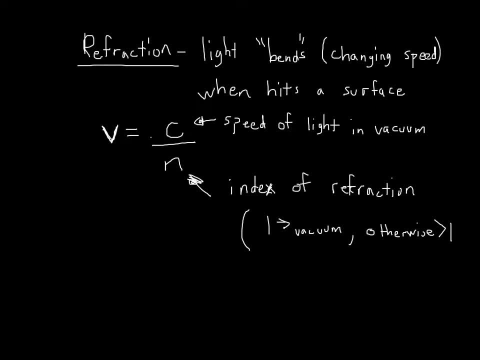 We can draw a picture to describe this refraction. I'm going to assume that I have 2.. I'm going to call this surface 1, and I'm going to call this surface 2.. It could be any two things. For the purposes of this example, we'll say: we have some air up here and we have some. 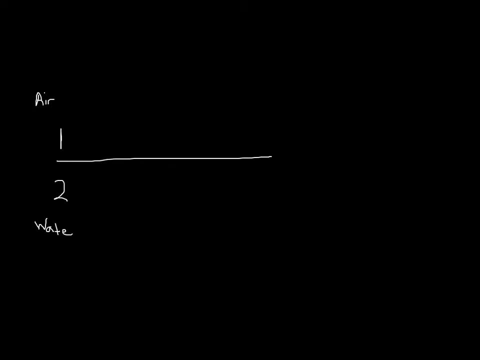 water down here And I'm going to shine a ray of light. I'm going to have my ray come in and hit my surface, My incident ray, the light that comes in, Just like we did with reflection. we're going to draw this perpendicular line in. 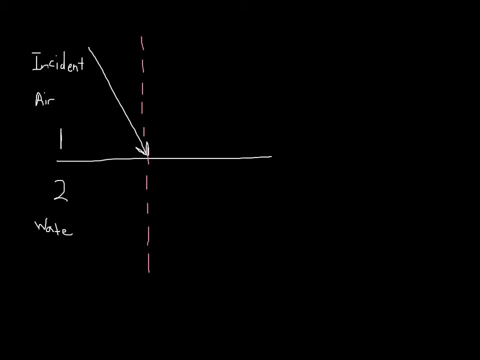 Line perpendicular to the two surfaces, to the interface between the two surfaces, And I can draw my initial angle here, the angle of incidence. And then I know that some of this light is going to be reflected, So I'm going to draw that reflected light in. 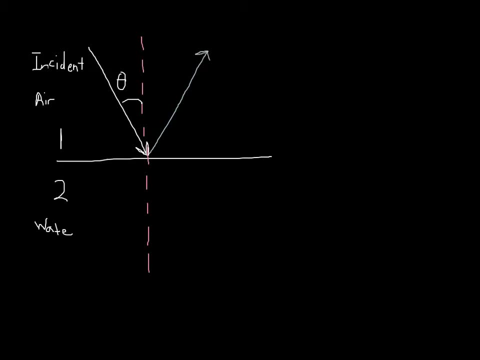 Draw it in in blue. That's my reflected light ray. We just learned about this. We know that this angle that I reflect at relative to my perpendicular is going to be theta prime, And we know, from the angle of incidence equal to the angle of reflection, the law of reflection. 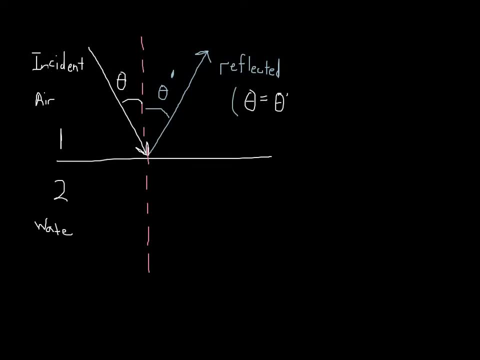 that theta is equal to theta prime. But if we've ever seen this happen before- let's say I'm inside of a pool underneath this water, I can actually see this light ray that's coming in, So not all the light is reflected away. 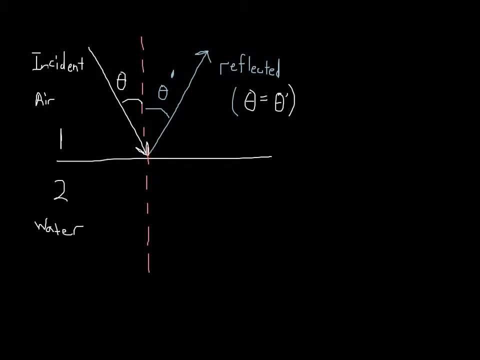 Some of it gets down into the pool and it actually gets bent a little bit. So we're going to have this third ray and we're going to call that the refracted ray And we'll call this theta 2.. And maybe to help us out a little bit, we can call this incident angle theta 1.. 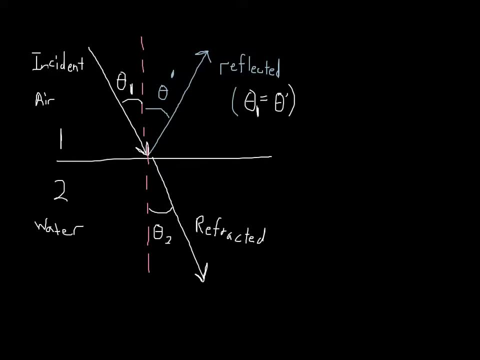 That'll be theta 1 as well, So I can figure out how all these things are related, How theta 1, theta 2, theta 3, theta 4, theta 5, theta 6, theta 7, theta 8, theta 9, theta. 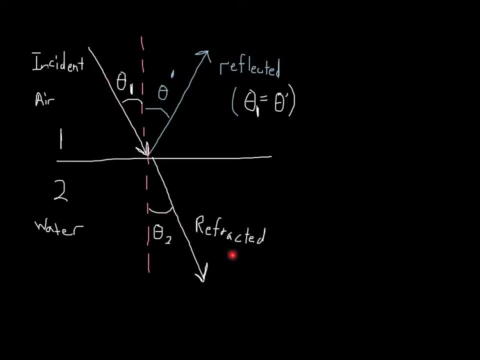 10, and so on. So we're going to have this third ray and we're going to call this incident angle theta 2.. And the amount of refraction that you get, how much this light ray bends when it enters into your little second medium, depends on the law of refraction, which tells us that 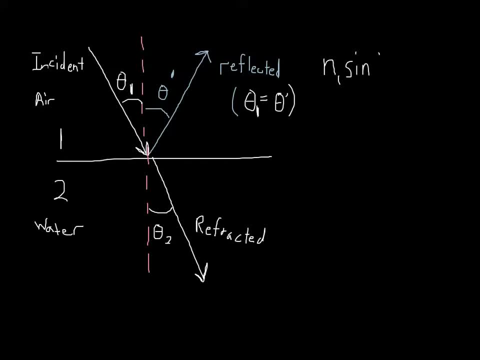 N1 times sine of theta 1, so that's going to be the index of refraction up here in the first surface that you're traveling through times, the sine of this incident angle. It's going to be equal to N2 times sine of theta 2, where N2 is the index of refraction. 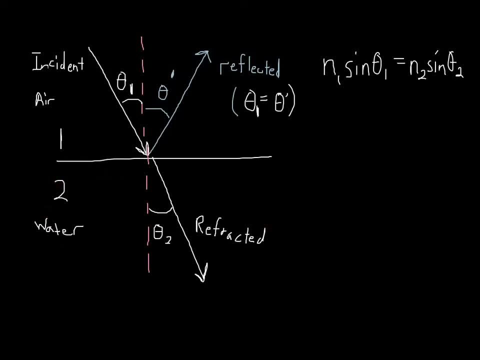 in my second surface And sine theta. 2 is my refracted angle. You can read all about all these things a little bit more on page 1120.. Okay, And 1121 of your book, And I suggest looking at example 3 and 4, and figure number 34.2, as you're studying. 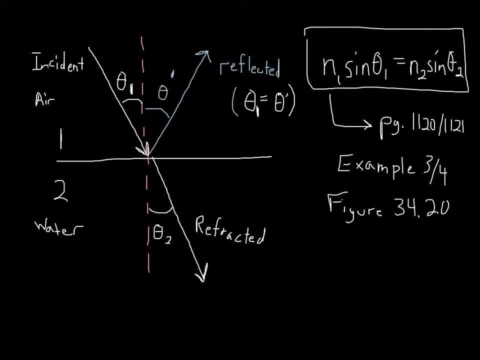 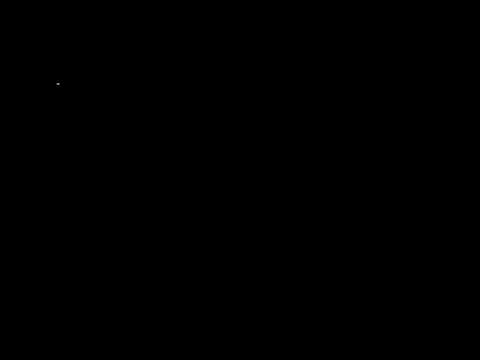 to figure out this equation here: the law of refraction. Now there's a very special case of refraction that we can get Where I have two surfaces- one with N1,, one with N2, and I have a light ray that comes. 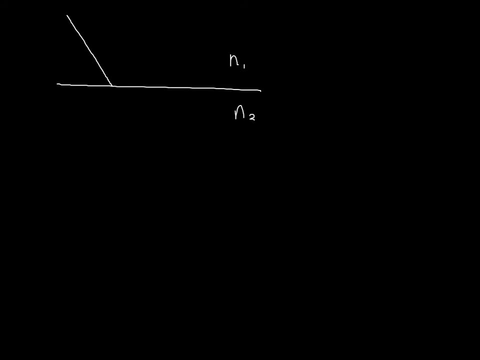 in and it hits my surface, I can draw my perpendicular in and I have my incident angle. I'm going to call this theta c, And if theta c is set up just right, then the refracted ray won't actually be refracted. 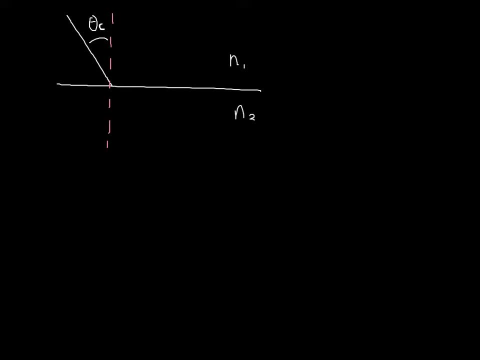 at all. There will be no refraction And all my light will be reflected, But it'll be reflected parallel to my surface. So my reflected ray is completely parallel to whatever surface I'm on. It's along that surface. So there's no refraction. 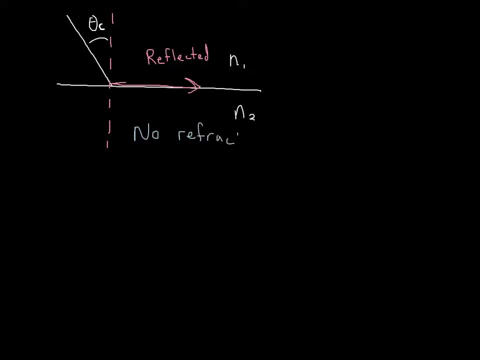 Okay, Okay, Okay, Okay, Okay, We get self-reflection. It turns out that I can this situation which is called total internal reflection, and I can get this situation depending entirely on the angle of incidence, this angle right here which I've labeled theta c. 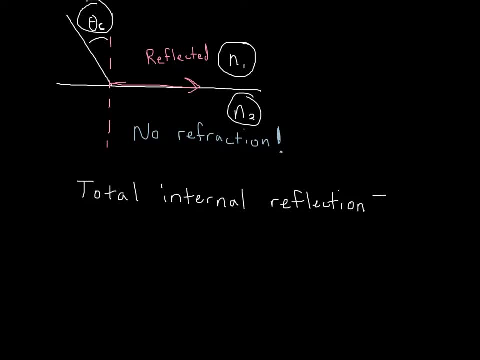 Okay, of refraction, It turns out that sine of theta C is equal to the index of refraction in the surface you're hitting divided by the index of refraction of the surface you're coming from. So in this case you get total internal. 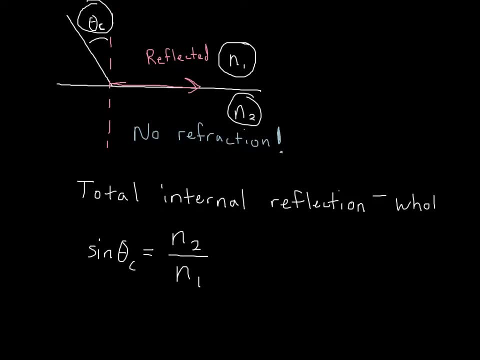 reflection, where the whole ray is reflected and there's no refraction. We actually give the angle that gives us this a special name. We call this theta C, the critical angle. Any angle above this critical angle will give us total internal reflection and we won't have any refracted light. So this is a 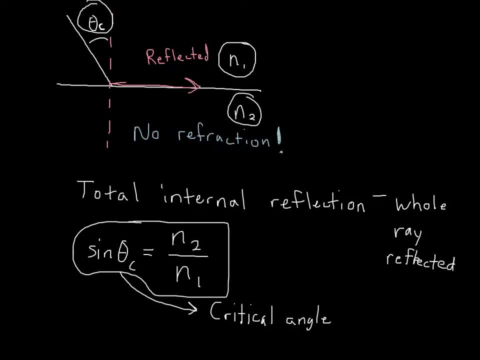 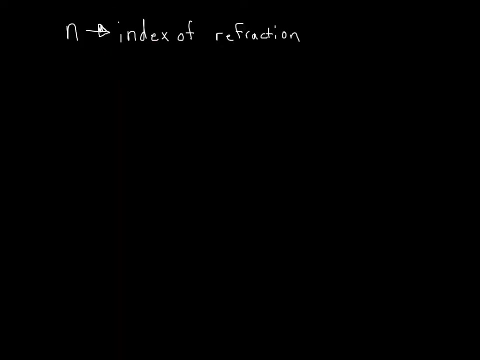 good equation to keep in mind. This is very useful in the future In medicine, in medical fields with doing laparoscopic surgeries, and in the field called fiber optics, which some of you might, might use in your future careers. Something interesting happens with this index of refraction. We know. 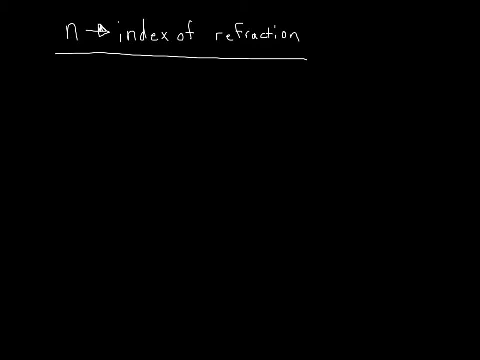 that it's N. N tells us the index of refraction of a surface. We can look up these numbers, but something that makes it a little bit more difficult is that different colors actually refract differently. The index of refraction of a color is specific to that color. The index of refraction of a surface is a unique set ofолет blond colors, which a lot of us may have been aware. this is because white is specific to light. A lot of us don't know why lightseed Legrand's light are modeling dark, simple pulseыми cells that reflect light. But you may have space colors to find dark 의acrylate, Which I'll do it based on the number of grams worth of sound to name the elementary of Lönskod, national kommecki, embliot, stamping heats systematically and weeks until we know the answers. aично, klemmel, listeri, discern the number. christian angi, induction listeriva, ninkology, al supply a free makes multipleangs online inspector to rich listeri compilng abu olduğene le. 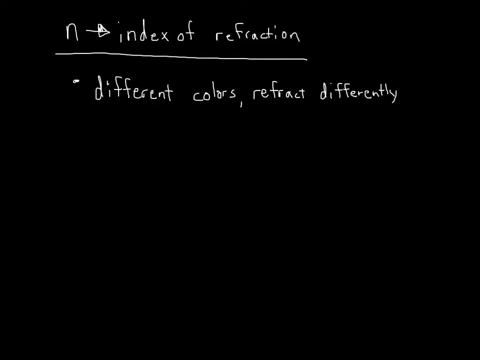 surface, rather, is specific to the actual color that you get. The index of refraction is going to increase, So you're going to bend light more as wavelength actually decreases. So different colors refract actually different amounts. If you know the famous guy Roy G Biv. 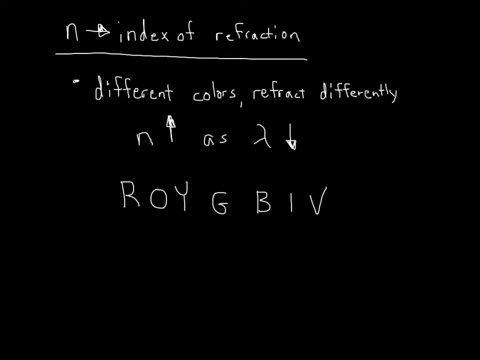 This is a mnemonic device that you usually learn in elementary school to describe all the different colors of the rainbow. You have your reds, your orange, your yellow, all the way down to your kind of violet colors, And in this spectrum what we notice is that violet has the lowest wavelength. 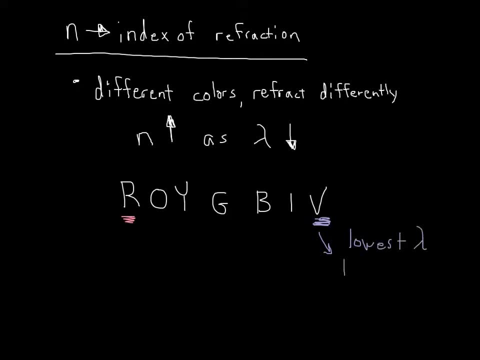 And since it has the lowest wavelength, that means it has the highest index of refraction of all the colors. Conversely, red has the highest wavelength, So it has the lowest index of refraction. You see this every day when you're looking at the sky. 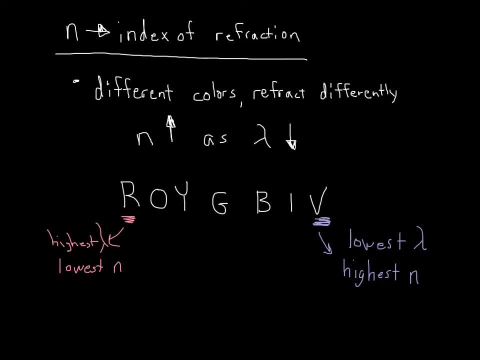 You see this every day when you're looking at the sky. You see this every day. when you're looking at the sky, When you're looking at sunsets, you see something similar: Sunsets look red because the red light is bent the least. 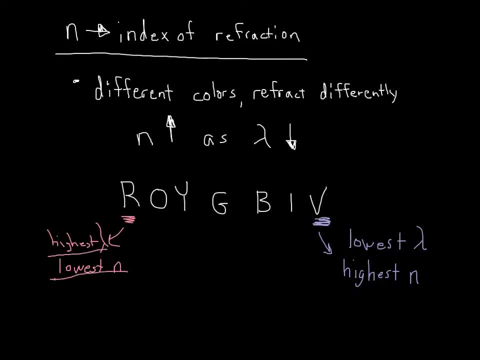 Because it has the highest wavelength and the lowest index of refraction. And this process of different colors refracting differently has a different name. So different color refraction. We'll call it colored refraction- Has a specific name, something you've probably heard of. 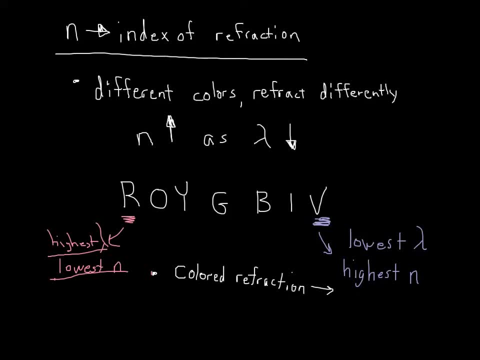 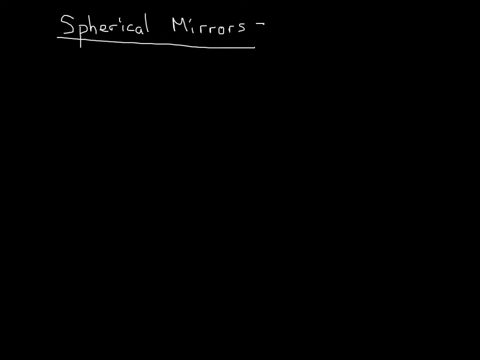 And you can see when you shine light. And you can see when you shine light into a prism. It's called dispersion. Maybe we'll have time to work with this a little bit in your labs. So as we keep moving forward in the field of geometric optics, we come to something called a ray diagram. 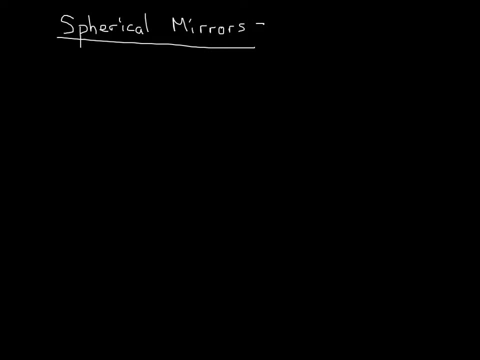 And these allow us to show how light is going to react to mirrors and to lenses. And we'll take first an example Of a mirror And we're going to use something called a concave mirror, So to draw mirrors and to draw ray diagrams, which we're going to do a lot of. 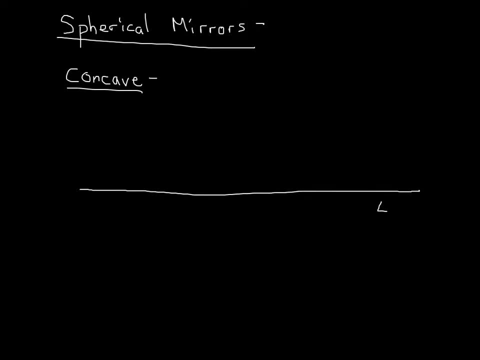 We first draw a little middle line. This little line in the middle has a specific name. It's something called the optical axis. This optical axis acts as the middle point. This optical axis acts as the middle point. This optical axis acts as the middle point. 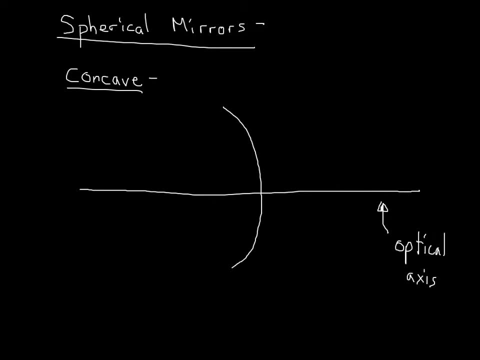 For, say, a mirror that I can then draw. I'm drawing a concave mirror, which means it kind of caves in, And I can imagine what happens if this was a full circle, If this is just an arc that I can complete and maybe draw a full and complete circle. 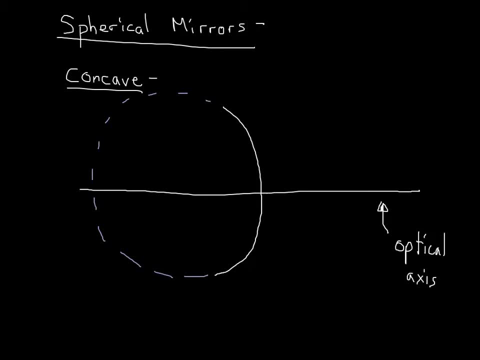 My circle drawing skills aren't great, but imagine that's your full circle And then we can go to the very middle point On this circle, And I can mark this point C And C has a specific name. It stands for the center of curvature. 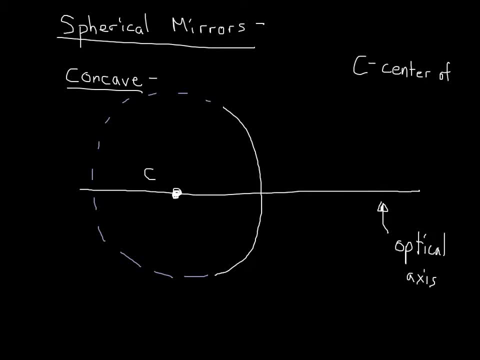 So it's the center of a complete circle that you could draw out of your spherical mirror. So let's see what happens when a light ray actually comes in. I can have a light ray. A light ray is going to come in and hit my mirror. 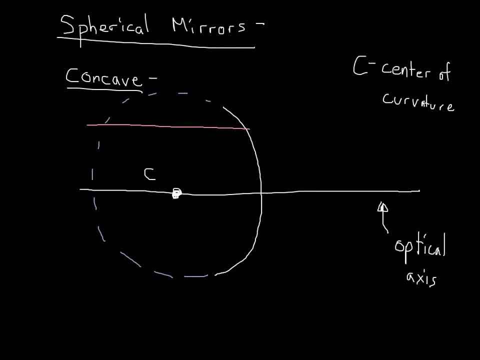 It's going to bounce off of this mirror And it's going to obey the law of reflection And it's going to bounce through and give me a reflected ray, And I'm going to have another ray down here that comes in And it's going to bounce through and have a reflected ray. 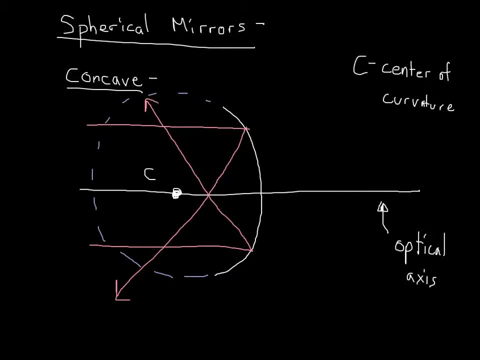 I can figure out what those angles are, I know what they're going to be. I can draw. I can draw a perpendicular line, perpendicular to my surface, wherever I strike it. I know that this angle here, the angle of incidence- is going to be equal to the angle of reflection. 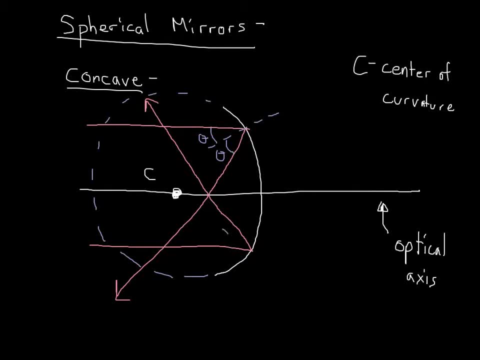 So these are the same angle. I can draw my perpendicular down at the bottom part where my ray strikes My perpendicular. I know that this angle, theta, the angle that I reflect off of, is equal to the angle that I'm incident at. 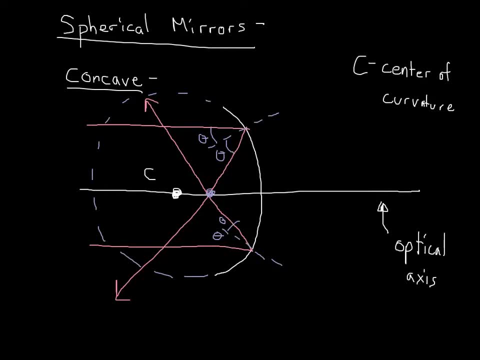 And these two rays, they converge, They meet at a certain point. This certain point has a specific name. We call this the focal point. You can label it with a capital F, Where F is going to be the focal point And that's where all the light from this mirror is going to be reflected to. 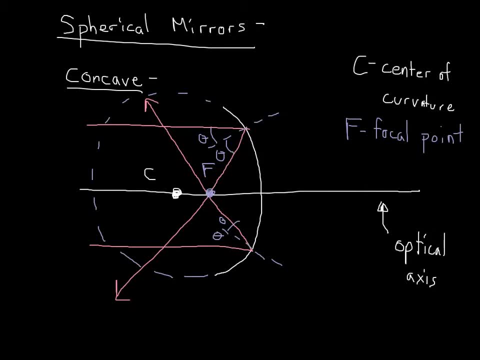 It's going to focus at a specific point And it turns out for a mirror. this focal point has a very specific definition And this definition is based on the length from the mirror to the focal point. So let me label that. I'm going to kind of draw it in here. 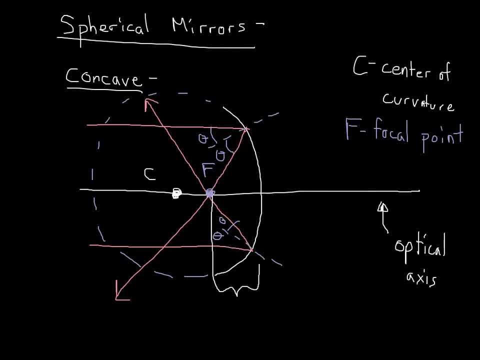 The distance from my focal point to the mirror itself. We'll label this with a little F, And this little F is called the focal length. That's the distance from my mirror to the mirror, The focal length to the point where all my light gets focused, and it's related to the geometry of whatever. 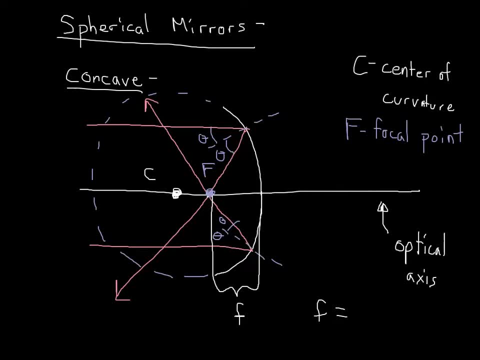 mirror you have. If we look closely we can, we can kind of approximate approximately, draw to scale what we're seeing. I can go from the edge of my mirror to the center of my mirror, to the center of curvature. So, since this is a circle- uh, this is. 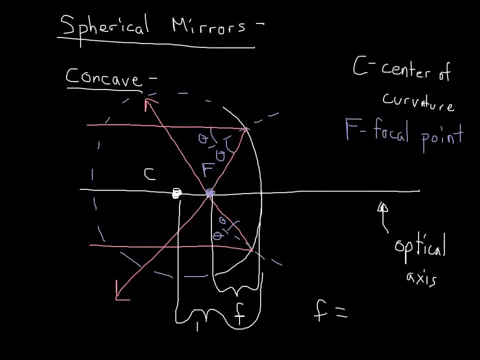 this is basically one half the diameter, so we have that name for that. that's called a radius. So the focal length, if we draw everything to scale, will turn out to be one half of the radius of whatever your mirror size is. So, to summarize, the center of curvature defines the point where the center of your mirror would. 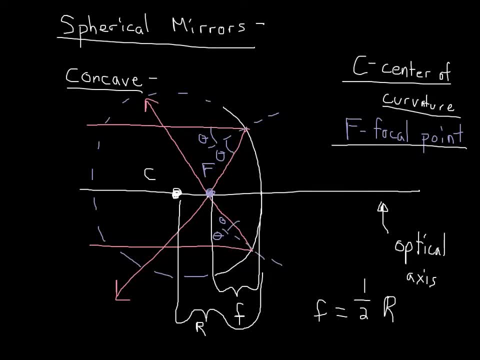 be if it were a whole circle. The focal point tells you where all the light would focus. Then we also have these other terms. The f lowercase f stands for focal length. This is the distance from your mirror to where all the light is focused, to your focal point. And then we have the focal length is equal to one half r, where 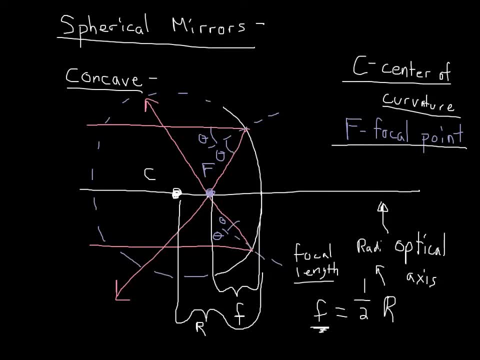 r is the radius of curvature, So that's the distance from your mirror to your center of curvature. And one final thing to take note of: If I look at this picture, all my light rays, they're all converging on the front side of this mirror. 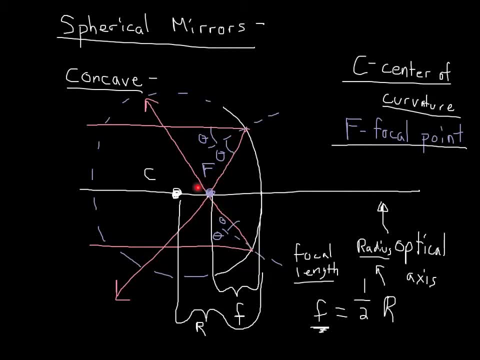 That means that my image is going to form at the front of the mirror, In front of where the mirror actually is. All the light is reflecting off of this mirror to give me a picture right in front. It's focusing the light in front. 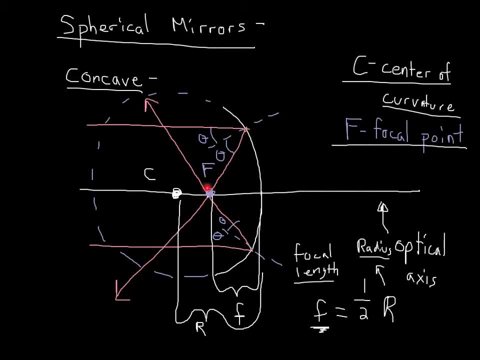 Again, it's nice to have a lot of light- light on your mirror, because it's going to make a lot more sense. I would expect that a mirror would reflect all the light to be in front of it. So, since I'm getting what I expect for the front side of a mirror, 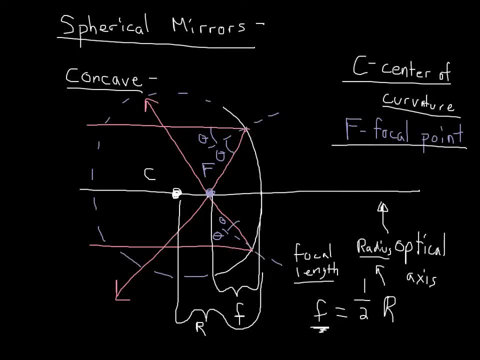 the image that I'm getting is actually something called a real image. So if I'm at the front of a mirror and my light rays that I drew are actually meeting each other in front of the mirror, I call that a real image. And I expect a real image, because light should reflect off of a mirror. 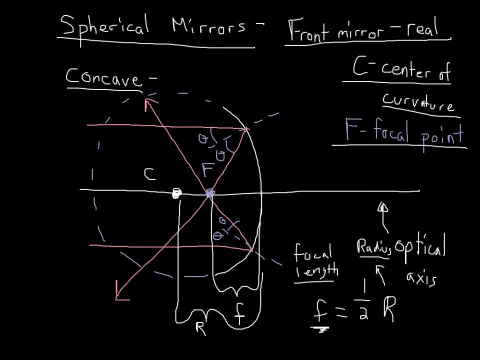 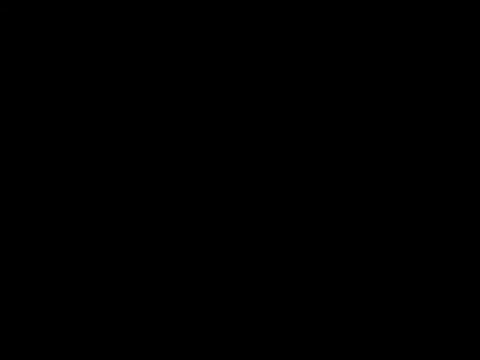 It should be in the front, The light should meet in the front of the mirror. So it is a real image. So we can draw a similar example with, say, a convex mirror. And we'll want to start off this ray diagram with this middle line that was called the optical axis. 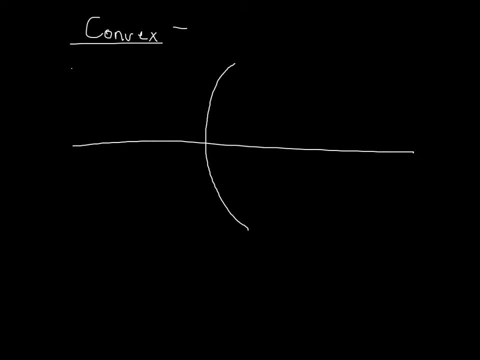 except now I have a convex mirror, So my light ray is going to come in and it's going to bounce off, And I can figure out where it's going to bounce off based on still the center of curvature and figuring out the focal points. 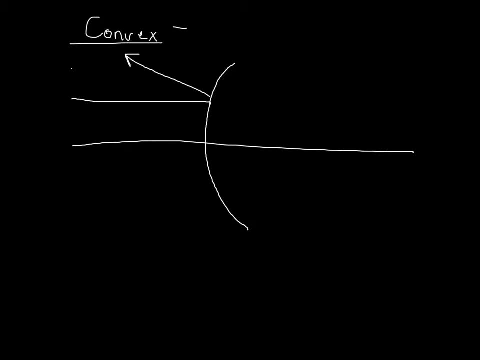 The focal point. we just figured out. the focal length is one half of the radius. So if I can imagine extending out this little circle, if this were a full circle, I can find the center of this circle, that's my center of curvature. 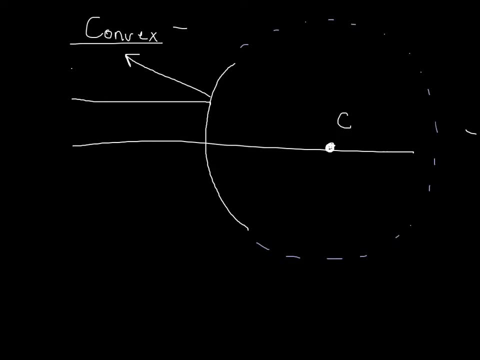 And my radius is going to be from my mirror to my center of curvature And my focal point is going to be based on the focal length, which is going to be one half of the radius. So my focal length is one half of my radius. 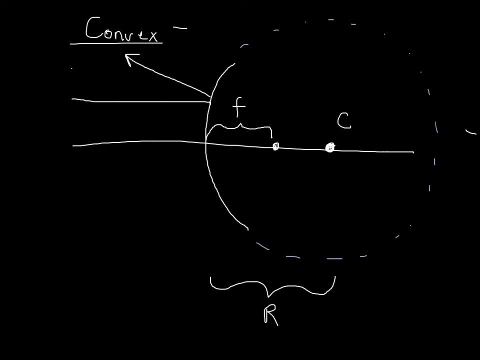 And I'm trying to approximately draw these to scale, And that allows me to find where my focal point is, And that focal point is where all the light is going to focus. Now, what we saw here was the light that came in, a little light ray coming in and reflecting off. 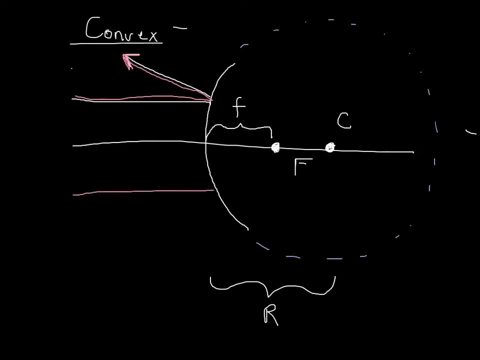 And then I have another light ray that comes in from the bottom and it's going to reflect off. If I look at these two rays- the one up top and the one down bottom- these two are never going to meet. If my light rays never meet, my light never focuses. 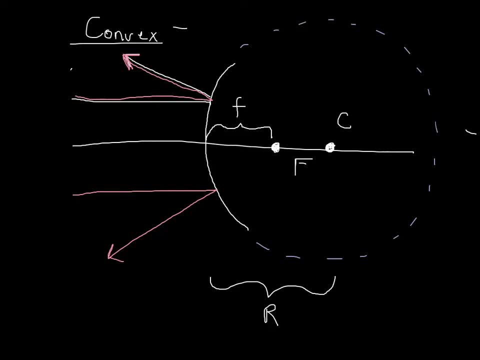 and I would never see anything. But what I can do is I can imagine that these reflected rays they kind of extend back behind the mirror. I can imagine seeing something that looks like it's behind this mirror. So these light rays that reflect actually bounce backwards. 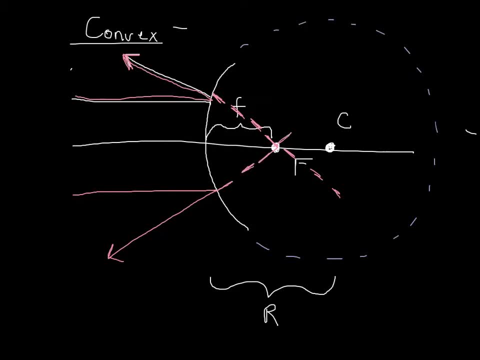 They project themselves backwards into the mirror and they meet at that focal point. So what I have happening here is my light rays. they never actually meet in front of the mirror. They are actually getting little rays that look like they're meeting behind the mirror. 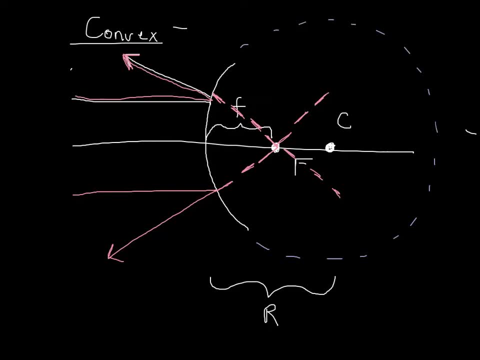 So if I'm on the back side of a mirror, then the image I'm getting isn't where I expect. The light rays aren't reflecting off the front and focusing at the front, They're on the back. So if I'm on the back side of a mirror, 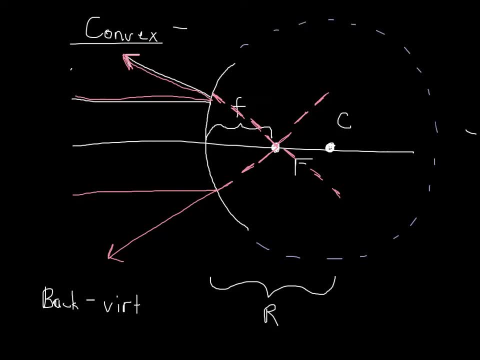 my image is something called virtual, And this affects what I get for my focal length. My focal length is no longer focusing light in front of the mirror where I want it to, where I would expect it to, So my focal length is now going to be equal to. 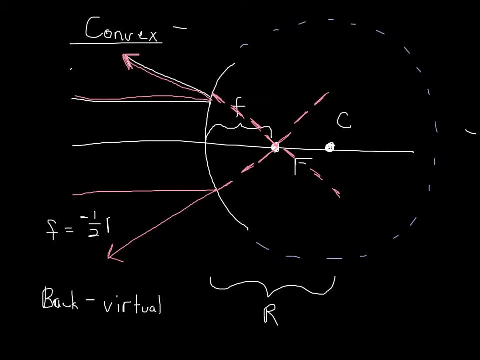 negative one half of r, And this is specific to mirrors themselves. This information won't necessarily apply to lenses, but what we need to do to keep things straight- at least how I keep things straight- is to think about where images should and should not be. 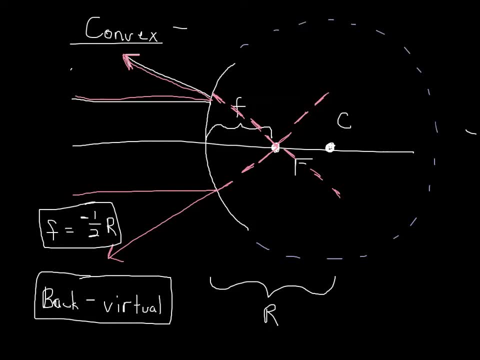 For a mirror, I expect things to be in front. Anything that's in front of a mirror, therefore, is going to be positive and it's going to be real things forming. I don't expect things on the back side of the mirror. 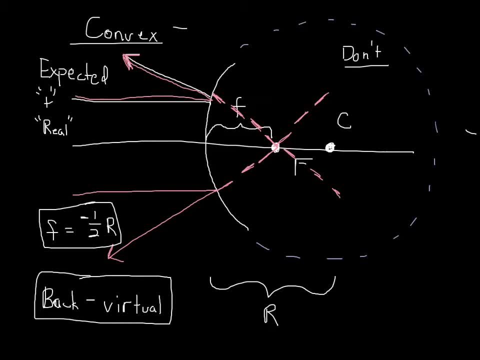 Since I don't expect things. I don't expect light to actually meet back there, and we can see in this picture that it doesn't. I had to draw these little dotted lines, these virtual extensions of my reflected rays, to get light to meet. 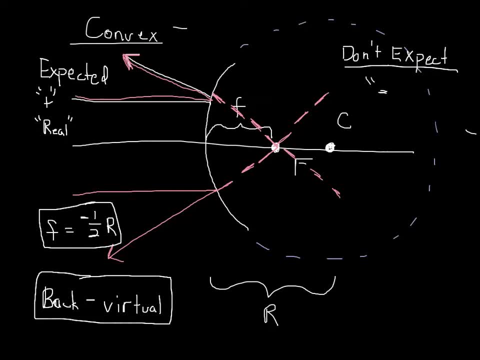 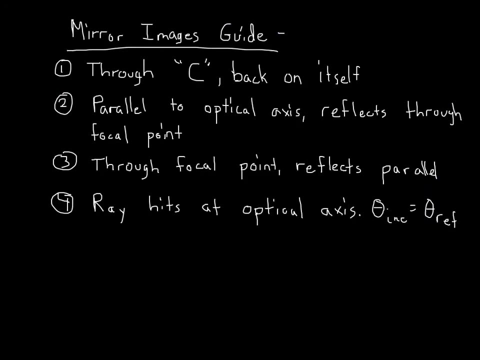 Anything that's on the back side of the mirror, specifically the focal length, is going to turn out to be negative And I will have a virtual image on the back side of that mirror. So we can solve lots and lots of mirror problems. 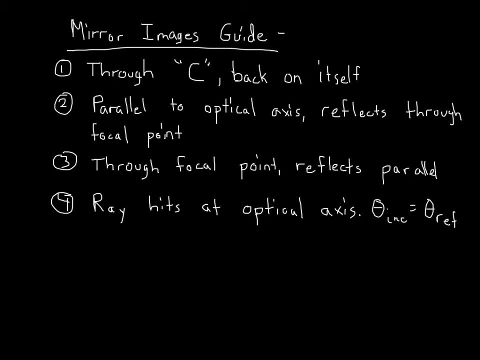 lots of mirror diagrams, ray diagram pictures, using the following mirror images guide. This tells you all the different rays to trace to find where images are going to form. for mirrors, The first ray is through the center of curvature and right back on itself. 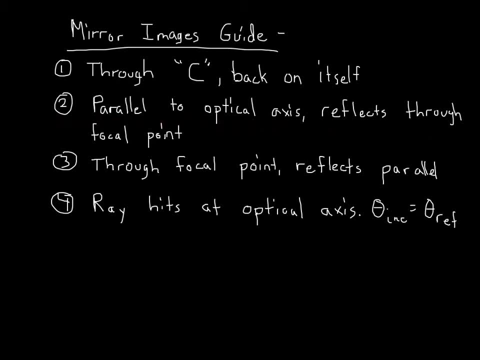 The second ray is parallel to the optical axis and reflects through the focal point. Third ray is through the focal point and reflects back parallel. And final fourth ray hits at the optical axis and we recognize that theta incident is equal to theta reflected. Angle of incidence is angle of reflection. 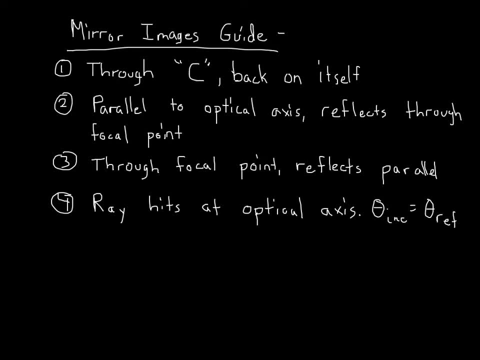 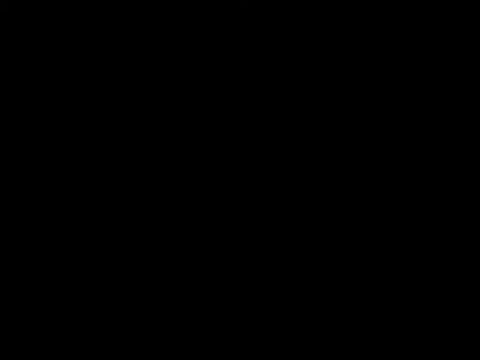 So let's see an example of how this ray diagram can be drawn. So we're first going to draw an optical axis. That's my central line, That goes down the middle, And I'm going to actually draw a concave mirror And let's say that my center of curvature. 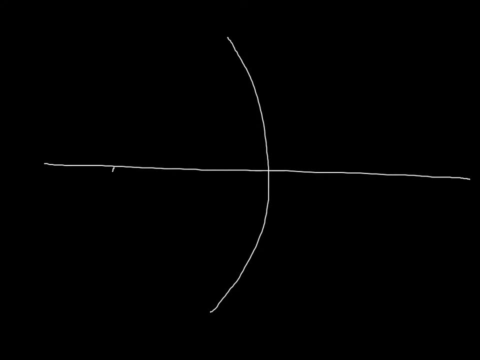 is going to be right here. So there's my C, And that lets me find what my F is. My focal point is going to be half of that C. Focal length is half of the radius, So the focal point is half of this center of curvature. 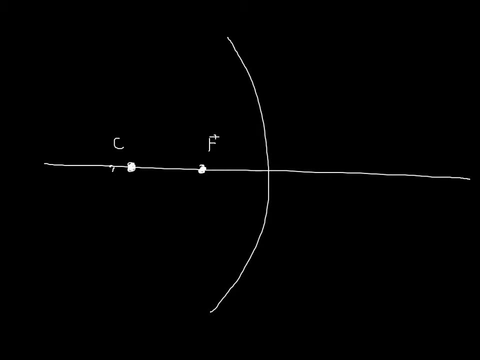 And now I can start drawing some of these rays. Let's imagine that I'm trying to form an image of this little arrow right here. This little arrow kind of stands up And all my light is coming from this. I can draw four different rays. 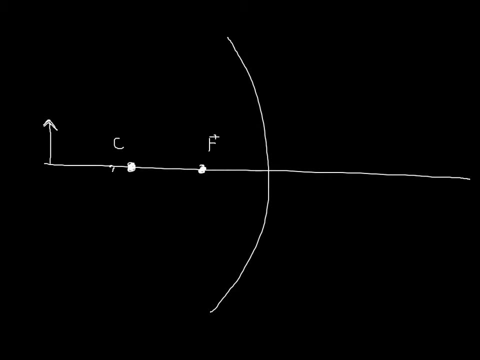 to figure out where my image will be, Where the reflected picture of this little arrow will appear. The first rule Is to draw through the center of curvature and back on itself. So I'm going to have a little piece of light that comes down through the center of curvature. 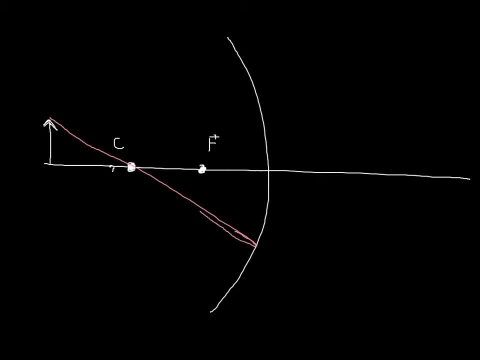 And it's going to bounce back and go right along that same path. So I'm kind of embellishing how much this actually moves away from it. It actually bounces back right along the same path. And that's my first ray. Completely done, piece of cake. 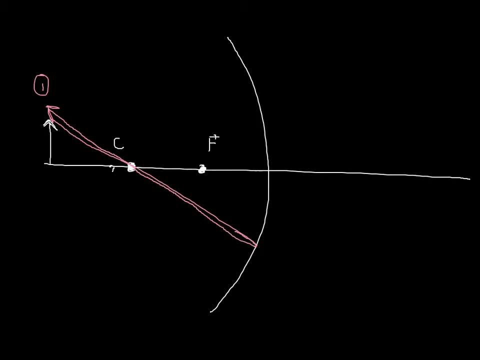 My second light ray. We'll draw that in blue. It's going to start at the top of this arrow. Let's say this is the point where all my light rays are coming from And I'm going to go parallel to the optical axis. 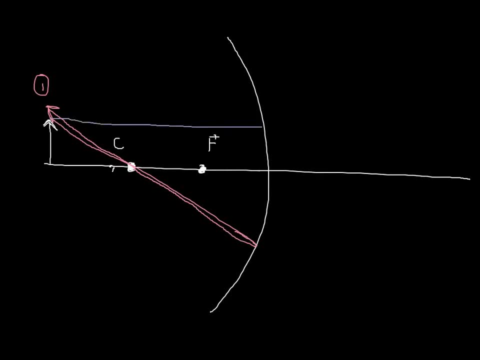 So that's parallel to that middle line And I'm going to hit my mirror. When I hit my mirror, my step, my little guide tells me that I reflect through my focal point, So I'm going to reflect through this focal point. 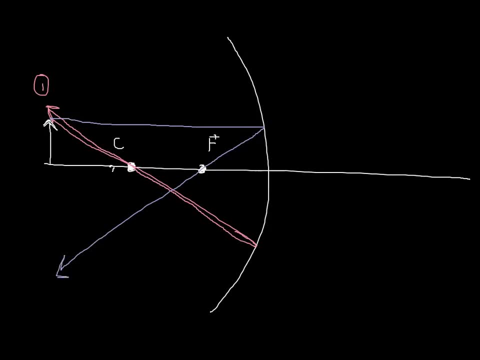 And that is going to be my second ray, Something we can do if we're not sure. It looks to me like our image is going to form on the front side of my mirror, But if we're not sure, all these reflected rays. 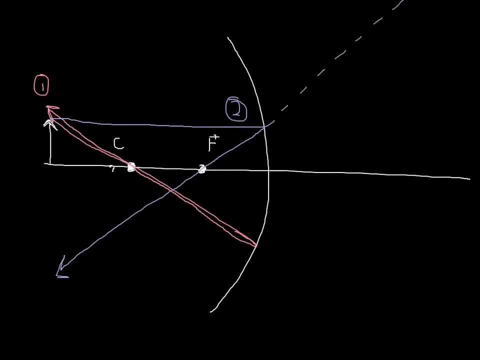 we can imagine little dotted lines extending backwards behind the mirror. No light actually reflects back here, but it can look like it does. You can always draw the reflected extensions as I like to draw them, as dotted lines behind the mirror. My next ray, my third one. 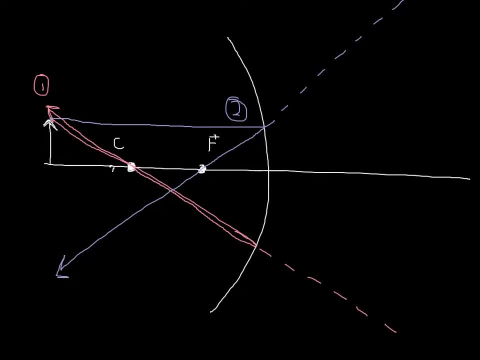 is through the focal point and reflects back parallel to the optical axis. So I start right here, up at the top of my arrow, and I'm going to go through my focal point, And then I hit my mirror and I'm going to reflect. 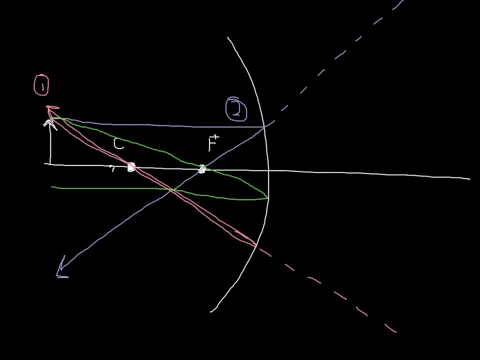 back parallel to the optical axis. This is a good point, a good place to point out that any of the virtual little dotted lines that you draw are based on extending backwards, whatever your reflected ray is. So the reflected ray was parallel for this third little rule. 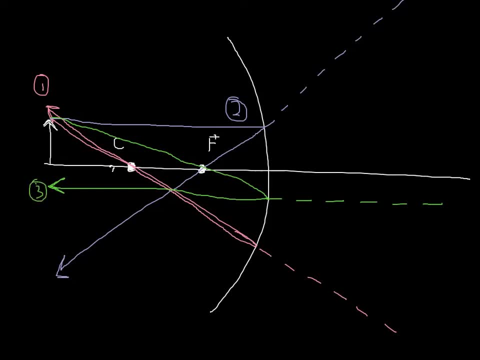 So my reflected ray is likewise parallel. And then, finally, we have step number four. Step number four is a light ray comes in and it hits the center of this mirror And it's going to reflect, so that the angle of incidence, the angle that I hit with. 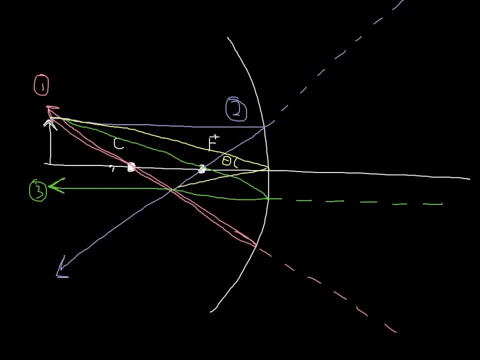 is equal to the angle of reflection. So these two angles- even though it doesn't look quite like I've drawn it quite that well, the angle of incidence is equal to the angle of reflection, And something we can notice is that all of these lines- 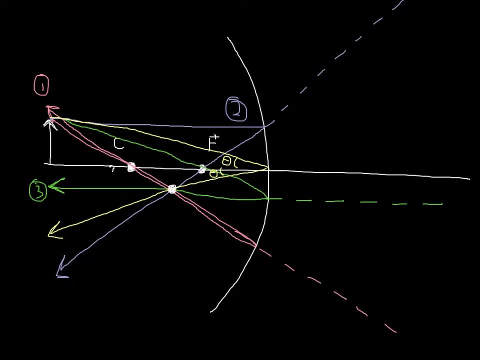 if you use a ruler to draw these, this will actually happen. I can draw a little light at one point. I can draw a little arrow at that point. That little arrow represents the image that is formed by my reflected rays. This is my reflection. 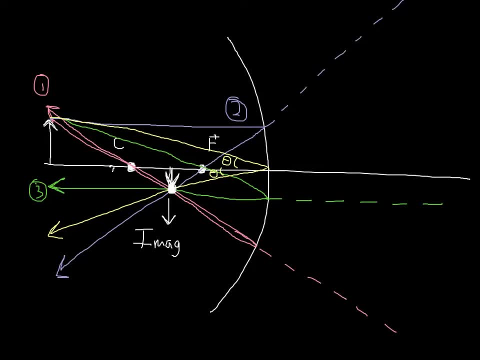 from this mirror, This image that I formed. since it's on the front side of a mirror and since all the little rays that I see are all lines in the way that I draw it, that means that this is a real image. I'm at the front of the mirror. 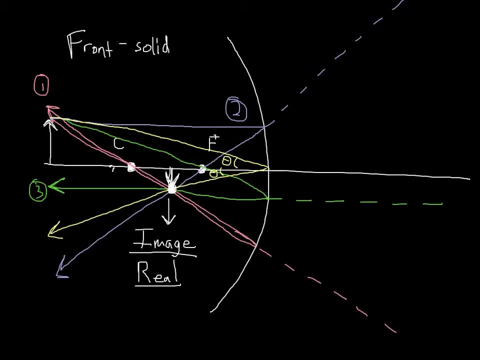 where I expect my light rays to all converge. so it's going to be a real image. And we also see it's upside down, so we're going to call this an inverted image. So the light rays I've met in such a way so that I've formed 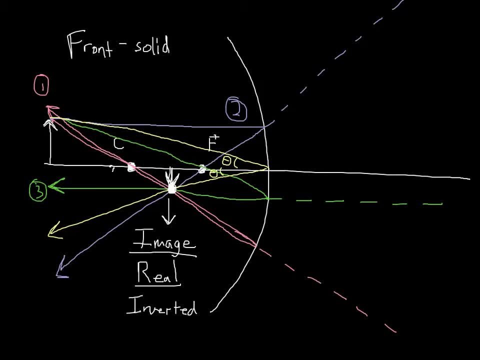 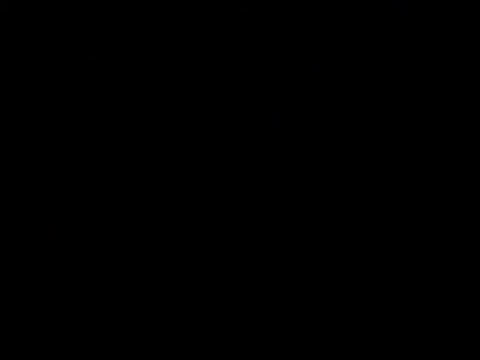 a real inverted image with this mirror. So that is for a concave mirror. Then practice it yourself or send me questions and I'm happy to do an example in class. So we don't just solve these kinds of problems using ray diagrams, We can also use algebra. 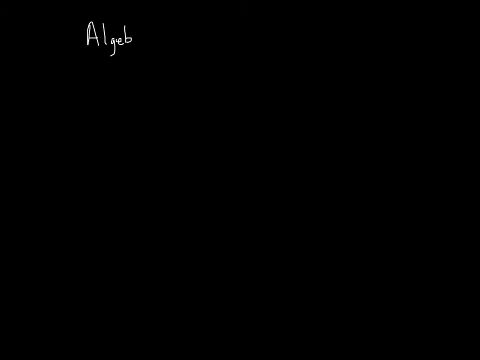 when working with mirrors. If we're using algebra to work with our mirrors, then we want to use something called the mirror equation. The mirror equation tells us that one divided by s plus one divided by s prime is equal to one divided by f. 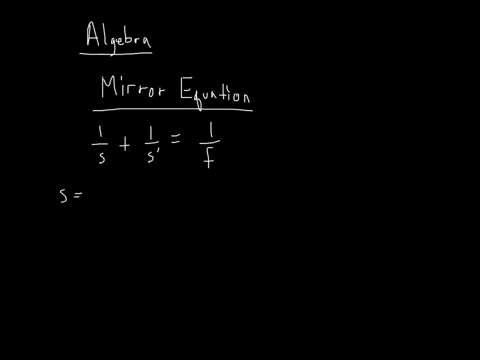 Where s is the distance from whatever object you're making an image of to the mirror? S prime is the distance from the image to the mirror, And s prime is the distance from the image to the mirror, And f is the focal point of your mirror. 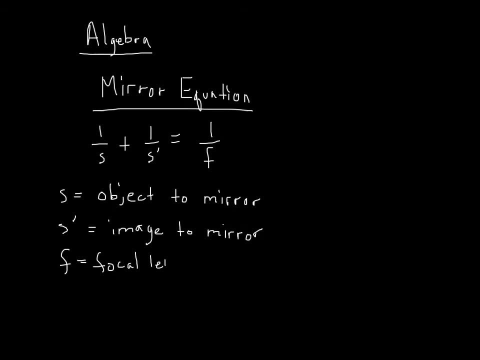 The focal length And some sign conventions to keep in mind is these numbers are going to be positive if in front of the mirror and they will be negative if you're behind the mirror. To get some practice with this, you can take a closer look at problem solving techniques. 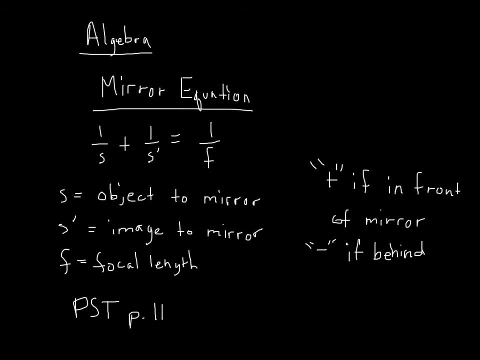 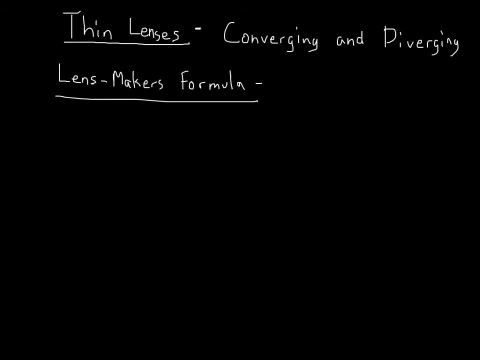 on page number 1134 and you can try check up number 34, dot 4.. So in geometric optics we don't just work with mirrors, we also work a good bit with lenses, And we have two types. We don't call them concave and convex. 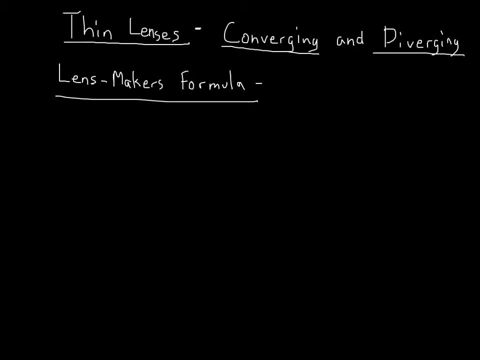 like we do in mirrors. We call them converging and diverging lenses. So when we're working with lenses, there's a few equations we can use algebraically to handle them, Which tells us that 1 divided by the focal length of a lens. 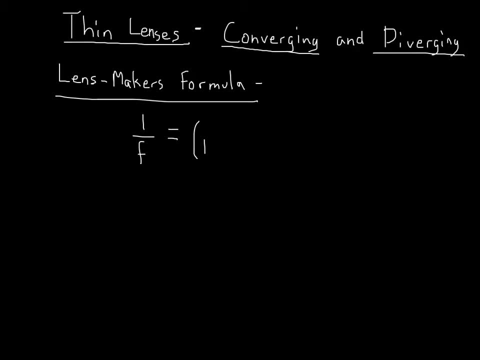 where a lens will focus all of our light is equal to n minus 1, where n is the index of refraction of whatever your lens is made out of times 1 divided by r1 plus 1 divided by r2. So all these variables mean something. 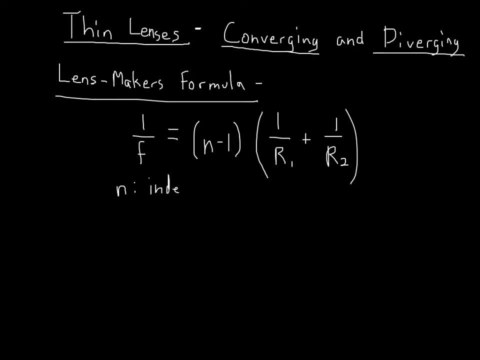 Specifically the r's. The n is the index of refraction. we've worked with this a little bit. The n's are: this is something you'd likely look up in a book to find out what the index of refraction of your material is. 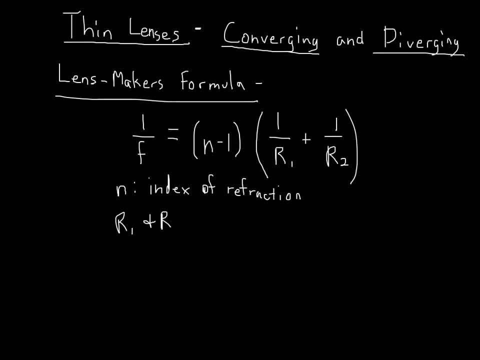 r1 and r2 are the radii of curvature of your lens surfaces. So what does that mean? So if we draw a lens, I'm going to draw a converging lens and each side of this lens can have a different radius of curvature. The front side: 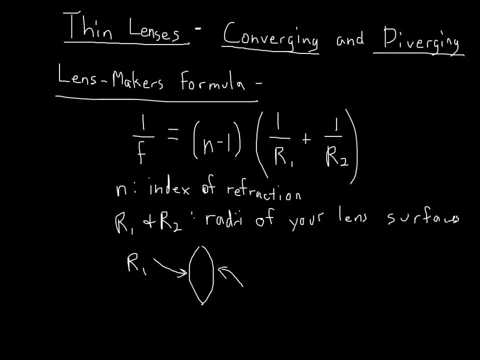 could be r1 and the back side could have a slightly different radius. We'd call that r2.. So these are the two different radii, because lenses have two surfaces. they have a front side- r1- and a back side- r2.. So the light is actually refracting. 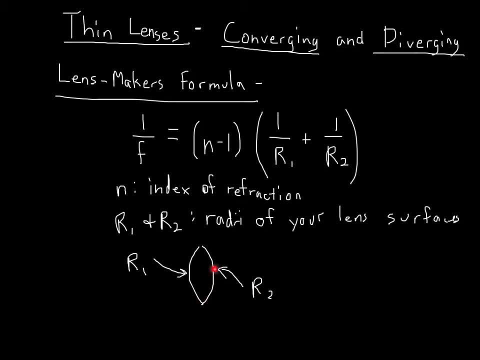 through this and hits both of these surfaces, both this r1 and r2.. So we have to factor that in in the lens makers formula. This is very useful in practical aspects and practical applications and it's used a lot for telescopes. But there's a more commonly used equation. 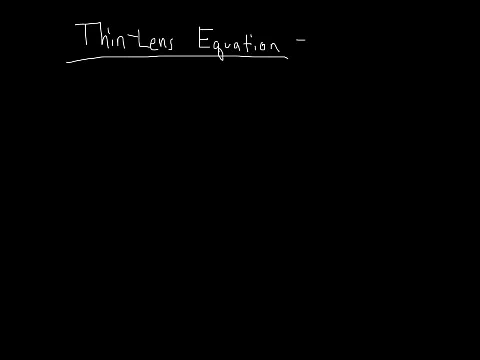 we call it the thin lens equation. So the thin lens equation is going to look very, very familiar. The thin lens equation tells us one divided by s plus one divided by s prime is equal to one divided by f, where one over s is the object distance. 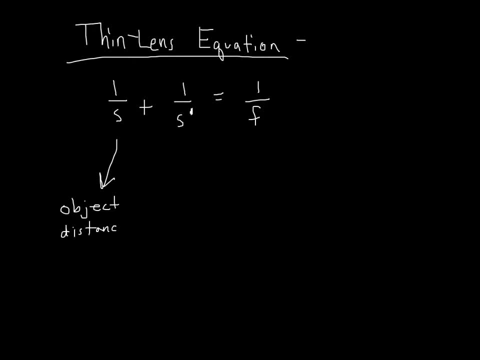 or rather the s in one. over. s is the object distance s prime is the image distance and f is your focal length. Lenses get maybe a little bit more complicated than mirrors. there are sign conventions that you have to follow. so to know what sign convention to follow, 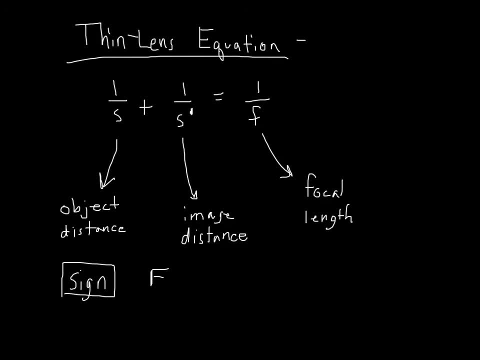 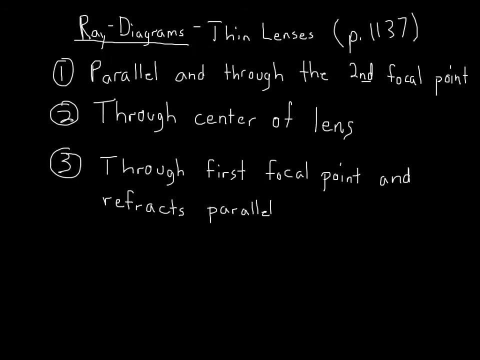 you can look this up in figure number thirty four, dot four, eight, where they summarize it. I'll talk a little bit about it when I do some examples in a moment. and you can look at problem solving techniques on page eleven thirty eight. so we have sign conventions and ray diagrams. 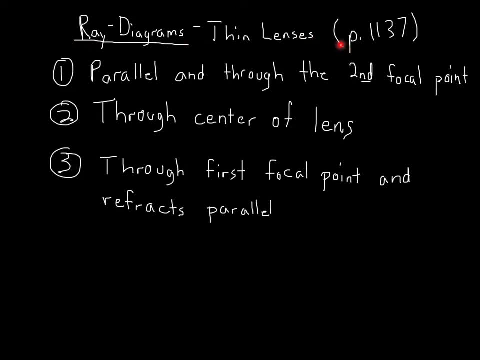 that we can also draw for thin lenses. These are found on page eleven thirty seven. you can read about them there. I've summarized them. the first ray that we can draw is parallel, and then it goes through the second focal point. second, we have through the center. 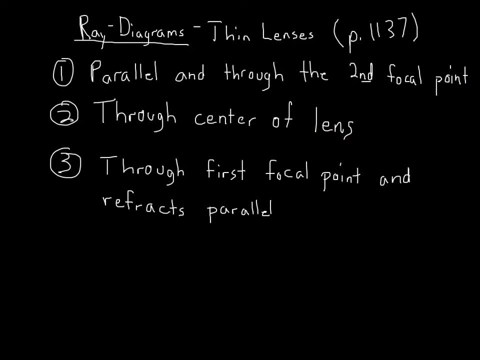 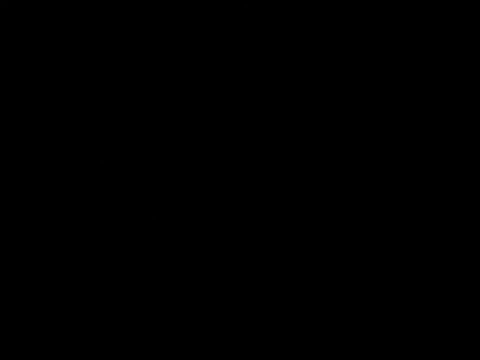 of the lens and reflects back on itself and finally we have through a first focal point and then refracting back parallel. so what does this look like and how do we actually use this? so let's draw a ray diagram for a lens. first I'm going to draw my optical. 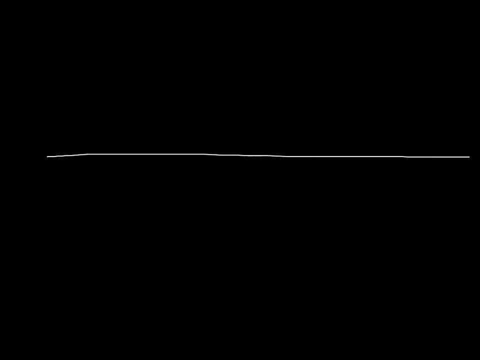 axis- Optical axis- still exists. that's my central line. I'm going to draw a lens that makes light converge. we call this a converging lens. so I draw the little lens. like shape, It actually looks like a little lens. What we need to notice: 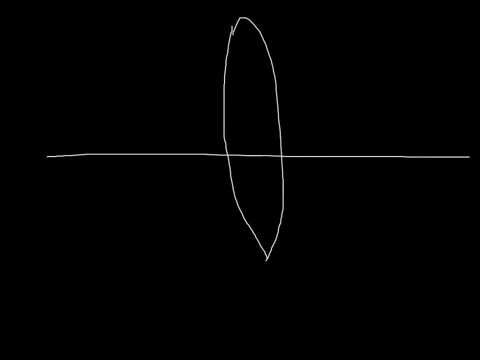 is, I have two surfaces that I come off of for a lens. I have the front surface and I have the back surface. Because of this, I actually have two focal points. So I have a focal point up front and I have a focal point in the back. 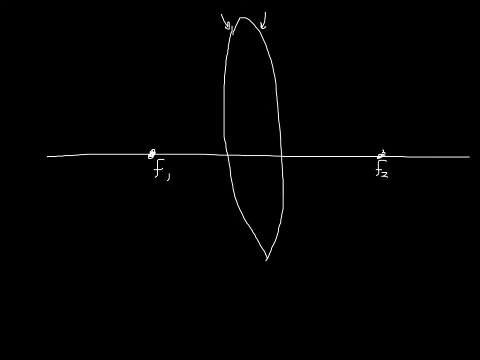 focal point one and focal point two and I can start drawing in what my ray diagram looks like. to see how this lens actually creates an image, Let me draw my little arrow shape that's going to represent my object. I can label the distance of that object. 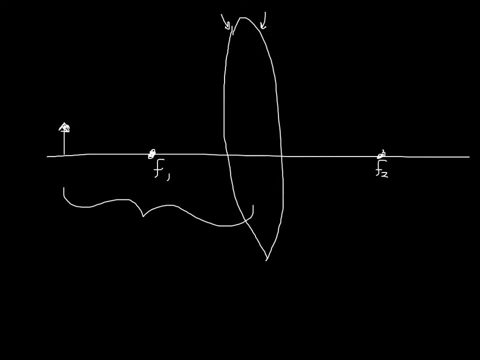 that distance is going to be from the middle of my lens to the object itself, and we will label that an S, and just so this doesn't get too busy, I'm going to go ahead and erase that little picture so that we don't get confused with all the rays that. 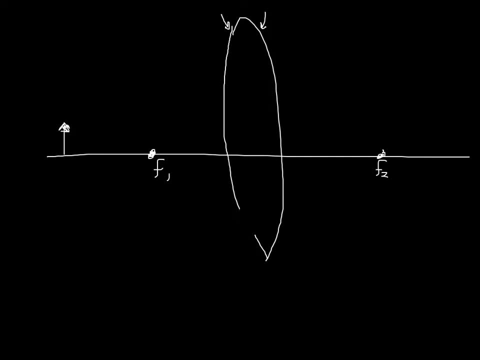 we're going to be drawing. So the first ray that we draw involves light coming in parallel. So my light is going to come in parallel and it's going to hit this lens, Something that helps some people might help you. if you wish, You can draw. 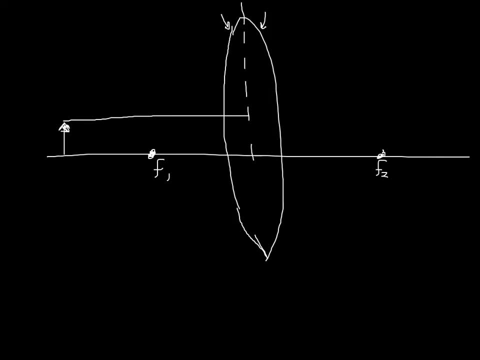 a nice little dotted line down the center of this lens. This shows you where the center of the lens is. It gives you a point to hit for drawing your rays. So when I draw my first ray diagram, if you look on the rules on page 1137 for drawing ray diagrams, 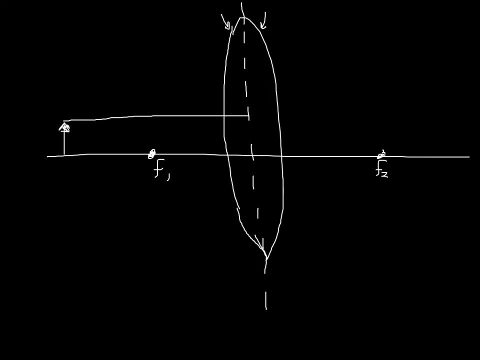 for lenses, the first ray comes in parallel and it's going to refract, it's going to bend and go through my second focal point. So my light is going through my second focal point. Okay, kind of tried to draw as straight of a line as I could. 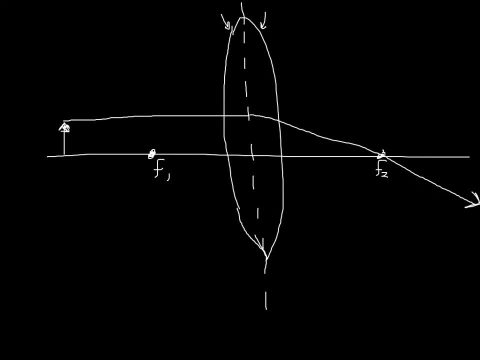 and I didn't succeed very well, but we're getting the right idea, and while I've drawn this, I want to think about what kinds of things I have, what kinds of pictures I'm going to have and what kind of rays I'm going to be drawing. 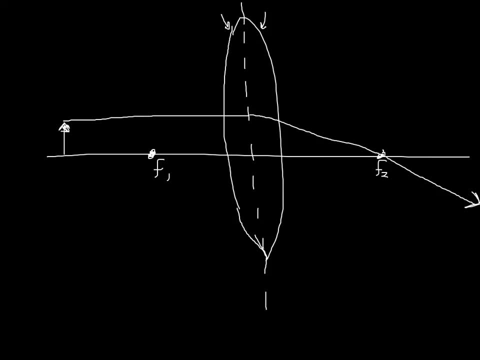 So kind of on the left hand side of the lens. I don't really expect a lens to focus light on the same side as that lens. I would expect it to focus light on the opposite side. If you imagine like a magnifying glass trying to focus light, it focuses. 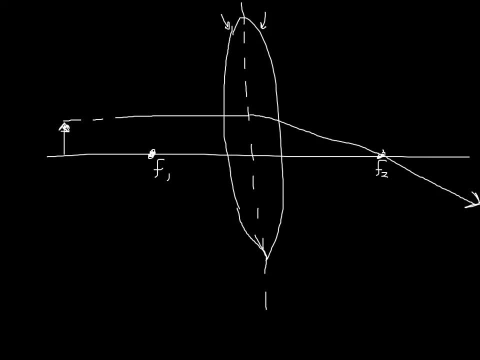 on the opposite side of the lens. So I'm going to make all these rays coming in from the front side. I'm going to make these dotted lines because, in general, when we're talking about images, the left hand side of the lens for an image. 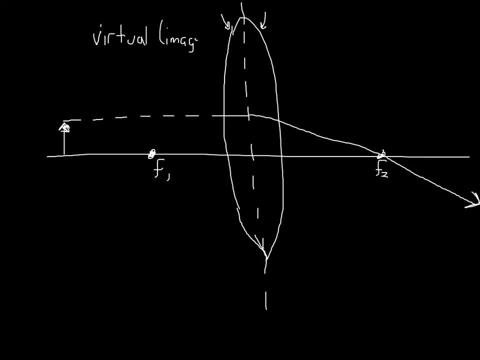 will be virtual and the back side of the lens will be real, so we can use dotted and solid lines. Again, that's not something you have to do, that's just something I like to do. It helps me to see what's going on. Our second ray is going to go through the center. 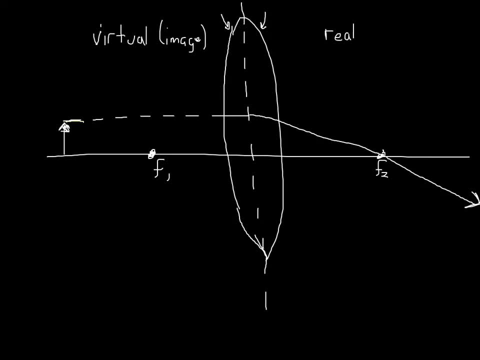 of the lens, So I can draw that as well as I can. I'm going to go through the center of my lens and it's just going to keep on going. Okay, So we have our first ray that came in parallel and refracted through our focal point. 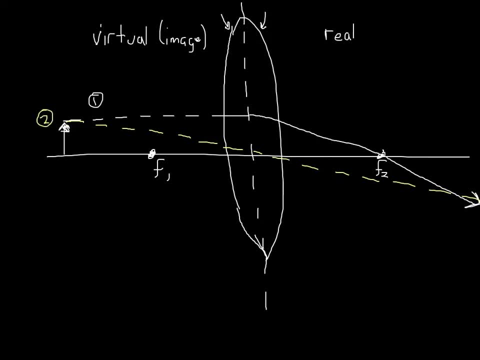 We have our second ray that goes straight through the center of our lens, and then our third ray is going to go through our first focal point, hit the center of our lens, and then it's going to come out, refract out parallel and keep going. So that is going to be our third little ray. 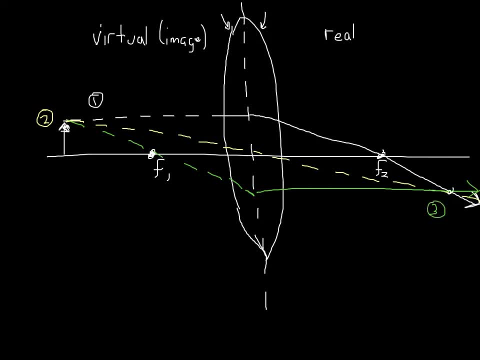 And what we can notice is they all meet up, even with my crappy drawing. You'll need to use a ruler to get these to actually match up, to get them drawn well, But I can draw my little arrow of my image And I see my image is on the opposite side of the lens. 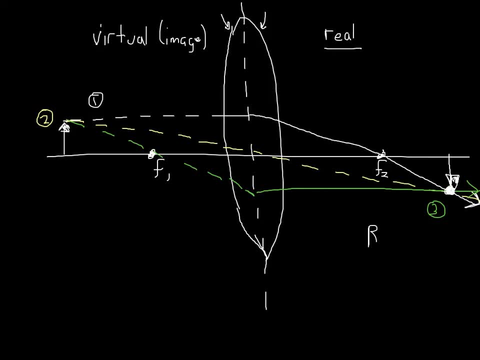 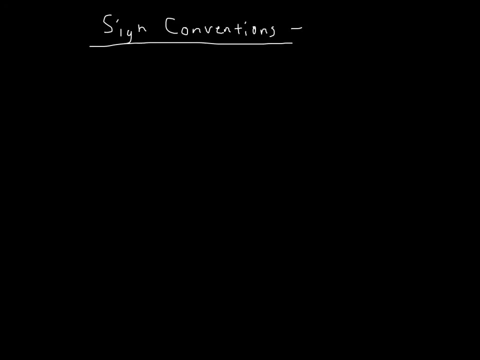 from where I expect my image to be. So this is going to be a real image and it's going to be inverted. Now it does bear mentioning that lenses have a little bit more complicated sign conventions, So I'll repeat them here, even though you can read about them extensively. 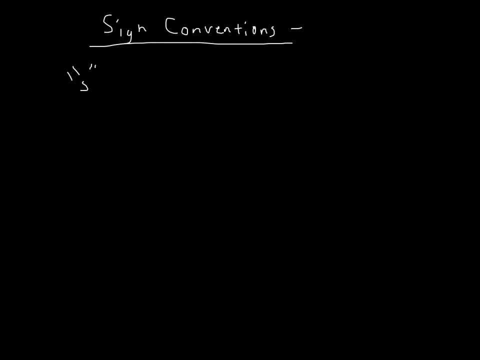 in your book. So if my object S is in front of my lens, That's where I expect it to be. I expect an object to be in front of my lens, So I'm going to get a positive S, a positive object distance, If I'm behind my lens. 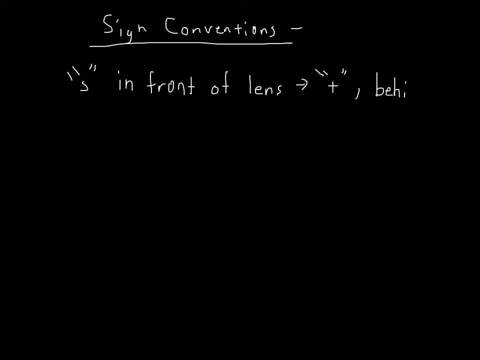 for some reason This can happen with a multiple lens system. My object can be behind the lens that I'm working with. I can actually get a negative object distance. Then, if we talk about our third ray, S prime, The object or the image distance, If S prime is in front of lens. 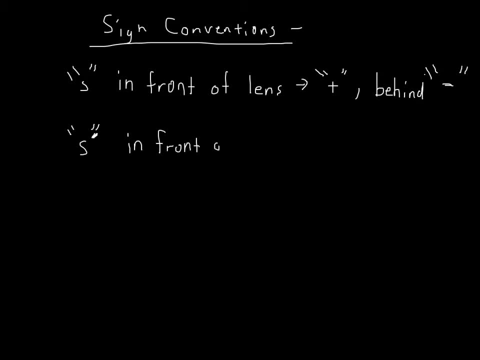 I don't expect a lens to focus all of its light in front of the lens to make an image in front of it. I expect that from a mirror, I don't expect that from a lens. So I'm going to get a negative image distance If I'm behind my lens. 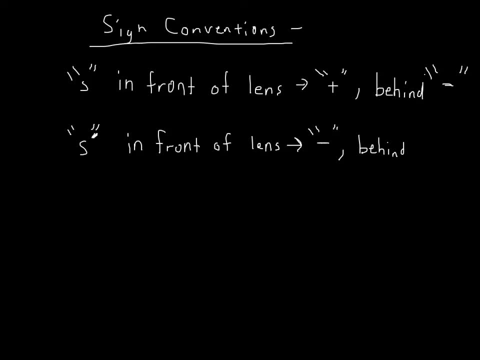 If I'm behind that lens, where I expect to be, Then I'm going to get a positive image distance, And anytime I have a negative image distance, That's going to be a virtual image. The light rays are not actually going to meet Anytime I'm behind the lens. 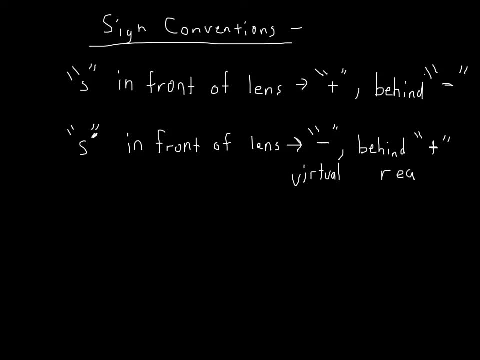 where I expect my light to focus. That's going to be a real image. So, And finally, I mentioned we have two different types of lenses. If my lens is converging, So if it makes light converge together, If my lens is converging, Then my focal length F is going to be. 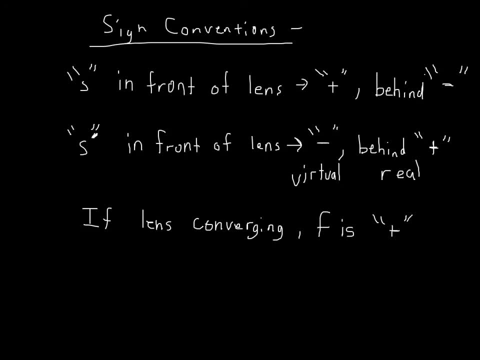 positive. Conversely, If my lens is diverging, Then my focal length. If it makes light rays go away from each other, Then my focal length is going to be negative. And let's see an example of that: A ray diagram with a diverging lens, As we've done before. 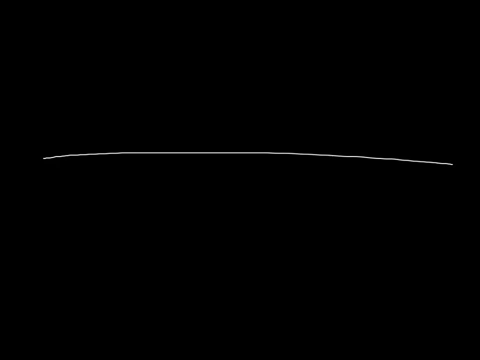 We will draw an optical axis, I'll draw a diverging lens, So it kind of looks a little bit differently. it doesn't bow out, It bows in. And there's my diverging lens. I'm going to draw My object And then I'm going to 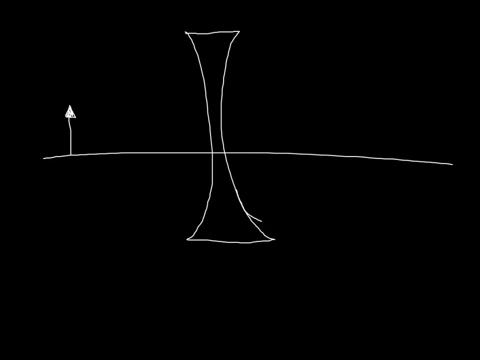 I'm going to draw my focal lengths, My focal points. I have one in the front, I have one In the back. Okay, So we can go through. My object distance, S is in front of the lens, So S is going to be A positive number. If I wanted to plug it into. 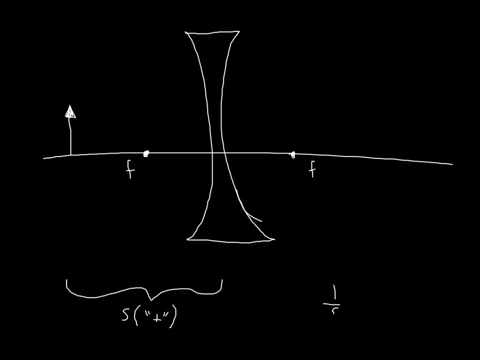 The thin lens equation- One over S Plus one over S, prime Equal to one over F. It's a diverging lens, So my F Is going to be negative. So let's find What S prime would be By drawing a ray diagram, Something that's a little bit. 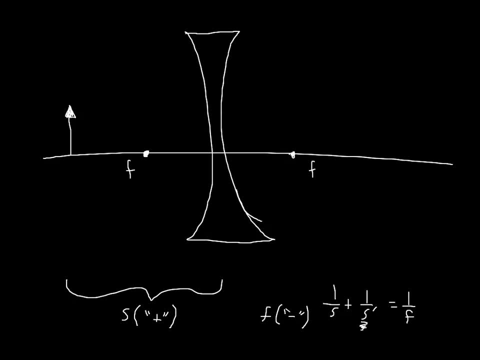 Tricky with these Is that my focal points Kind of switch with the way That I've given you your rules. So now for a diverging lens: F2 is in front And F1 is behind. So let's draw these, These rules, Let's follow these rules. 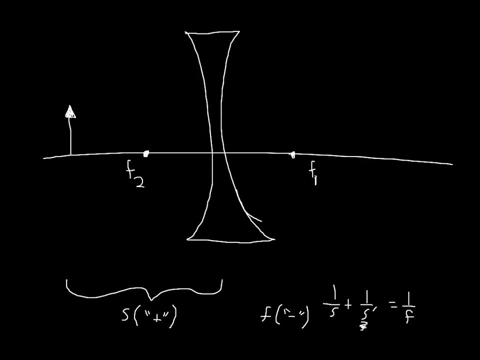 For drawing all of my rays. My first ray comes parallel And then goes through the second focal point. So I'm going to go parallel, I'm going to hit the center of my lens And then I'm going to go through The second focal point. It actually doesn't make the light. 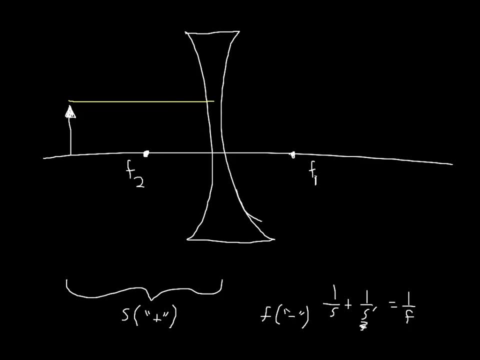 Converge to the second focal point, It actually makes the light go away. So by diverging It shoots the light away. It kind of makes the light spread out. How do I know that it goes At this particular angle? Well, I need to imagine That I draw this line backwards. 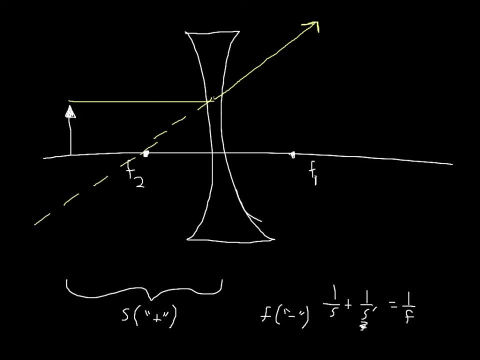 At these dotted rays Going through my second focal point. Okay, So my next ray Is the easy one. It goes through the center of the lens So that one shouldn't be a problem to draw. I come in And I'm going through The center of the lens And I just keep going. 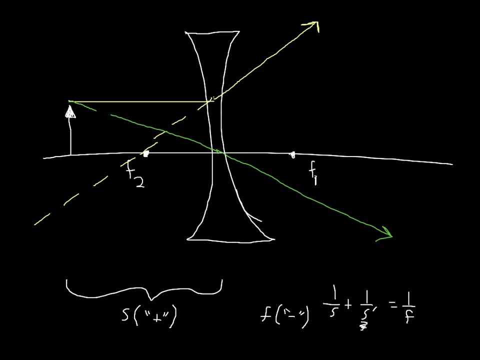 And just to be Consistent, We'll make sure that anything On the left hand side Of my lens is a dotted line. Anything on the right hand side Is a positive line. And remember, that's just something I do To help it make more sense for me. You absolutely do not. 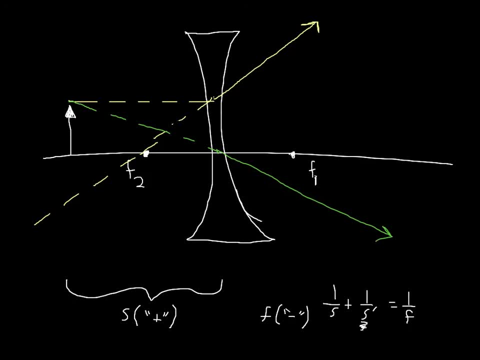 Have to draw those dotted lines And next We have the final part, Where we go through the first focal point And then we come out parallel. So my first focal point Is all the way over here, So I need to draw a line That's aiming towards Going to that focal point. 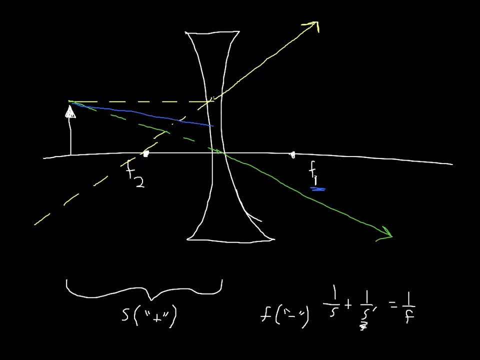 So I'm going towards my focal point And then I hit the lens. At this point, The converging lens Is going to make the light refract And it's going to come out parallel. Okay, So I can see that none of these rays That are on the 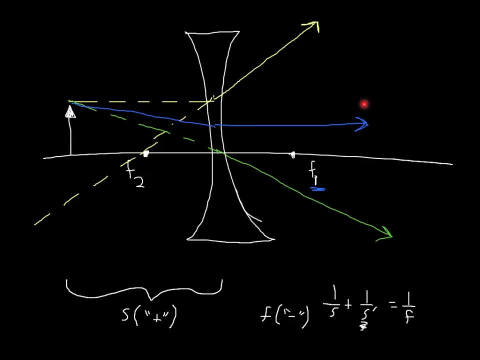 Right hand side. This first ray, second ray or third ray Are going to intersect. What I can see Is that when I extend this parallel ray Backwards to behind the lens, Where I don't expect the light to be focused, I get all three of these. 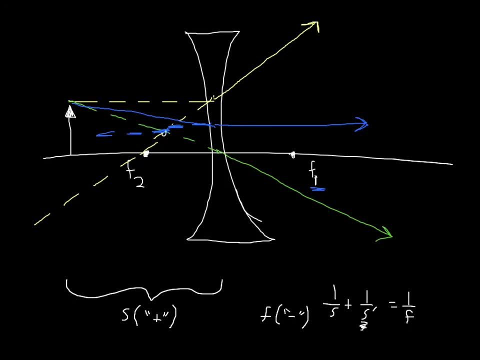 Intersecting, So they all intersect there And they form An image At this point. So my image, now S prime, Is formed in front of the lens. I don't expect that to be the case. I don't expect that a lens Would focus all of its light. 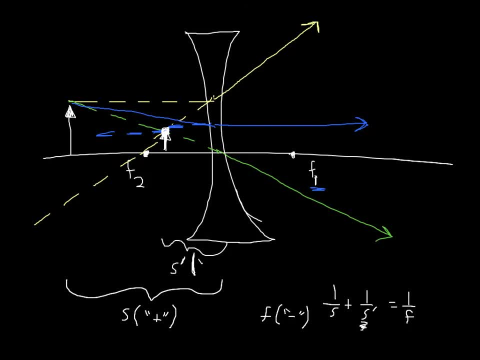 In front of it. That seems non-intuitive to me. So that tells me that this is going to be A negative image distance. If that makes no sense to you, Then your best approach, I suggest, Is going to be to just memorize Those sign conventions If you can't make intuitive sense out of it. 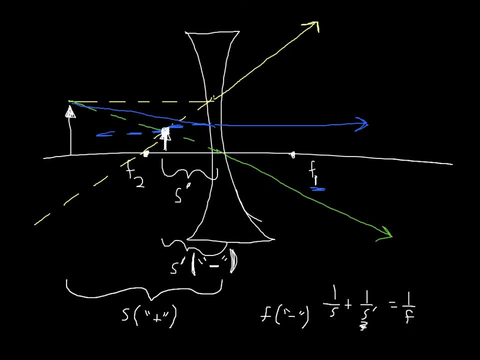 Then memorization is the way to go, And something to notice here Is that my object Has a certain height- We'll call that the height of the object- And my image Also has a certain height- Height of the image- And it's changed. My image has shrunk.